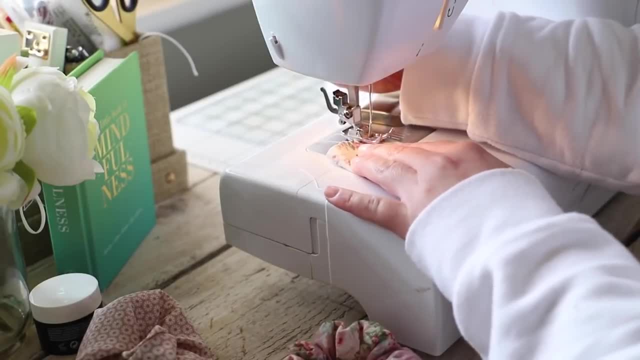 So I'm going to do a stitch from the top to bottom, and then you're going to pull it the right way Using your safety pin, which you're going to see how I do now, and that's going to make the casing for the elastic. 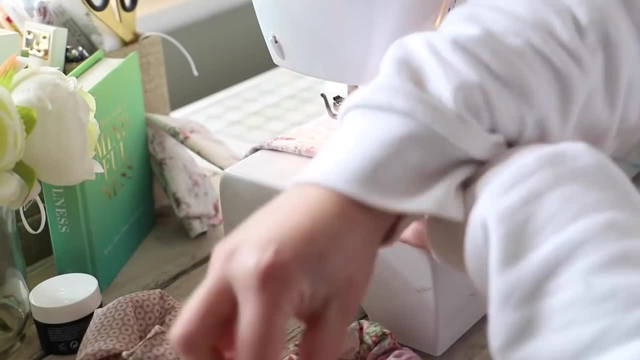 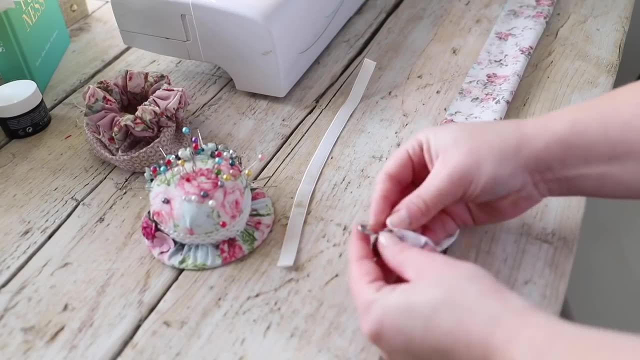 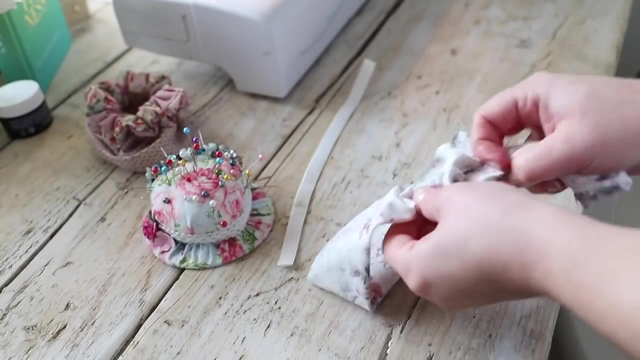 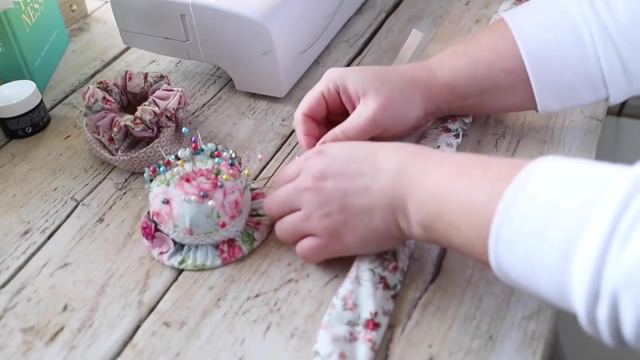 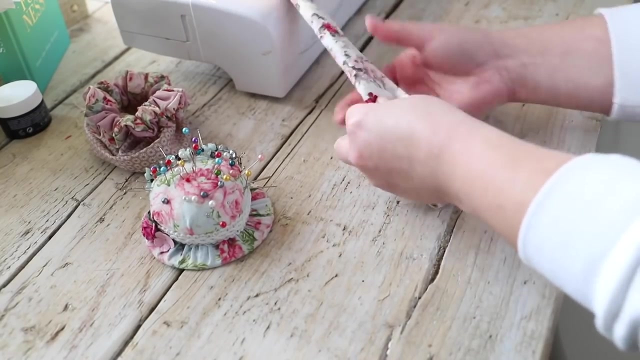 Using your safety pin again. you are going to thread it through the casing and make sure to have it in the right place. You're going to want to make sure that it's in the right place. Now hang on to the end piece, because when the elastic is threaded through and you see, 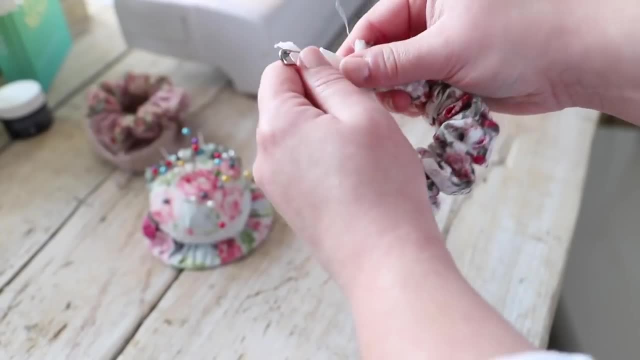 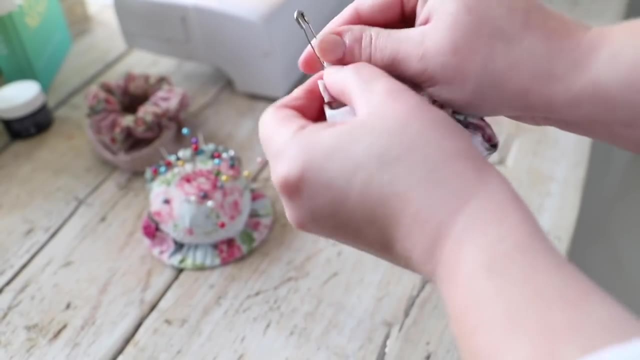 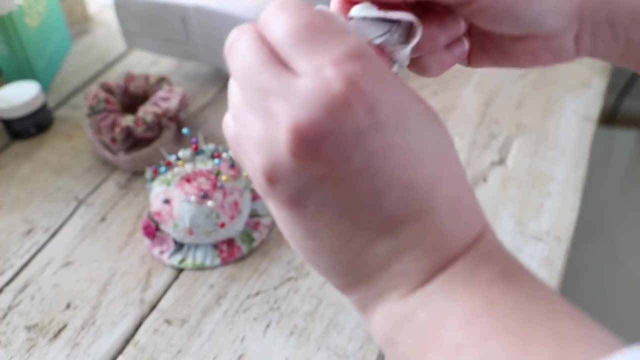 that the scrunchie is taking shape. you are going to tie a really firm knot with your elastic, and then the fiddliest bit of this project is just tucking the raw fabric in. so I just fold the raw fabric in against itself and then I do a straight stitch on the machine. 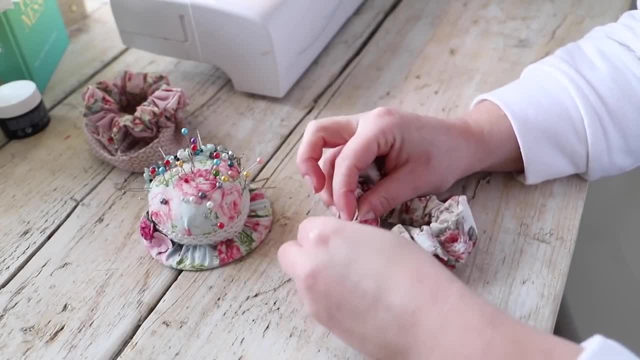 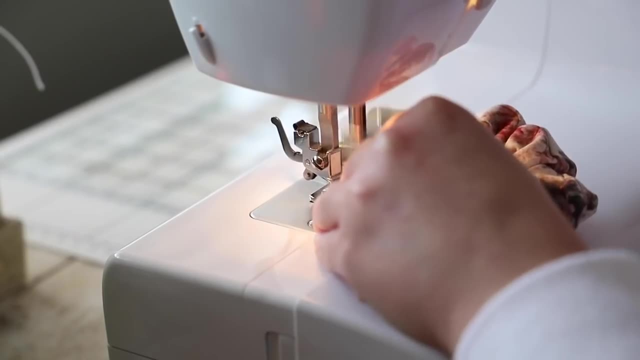 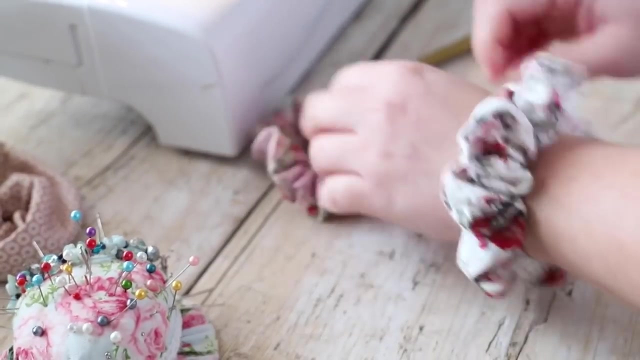 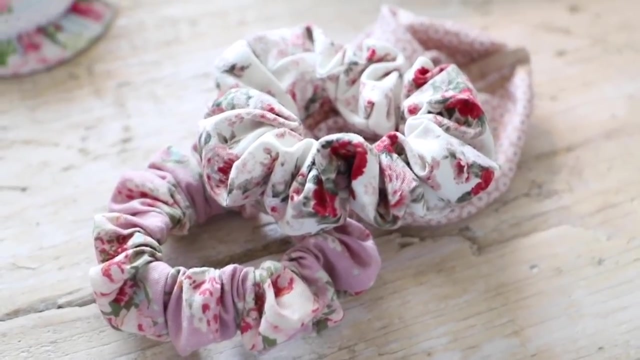 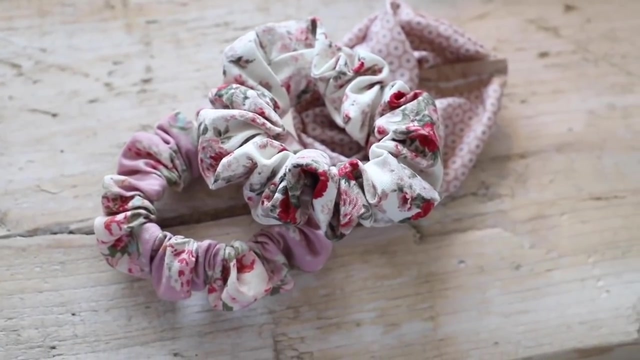 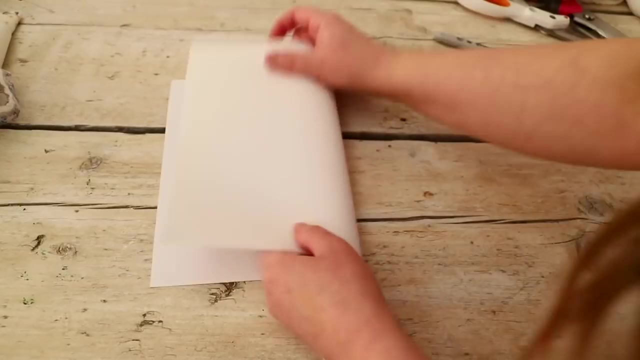 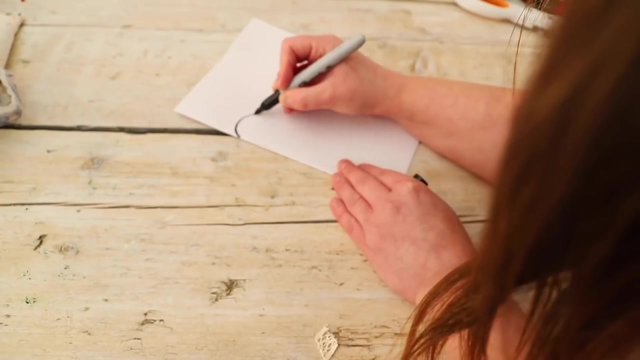 to secure all in place and the elastic, and then you have made yourself a scrunchie. We're going to make some coasters and I'm going to do a love heart shape. Now I'm sure you can download a love heart off the likes of Pinterest, but I decided I was going to attempt to do mine free-handed, By folding. 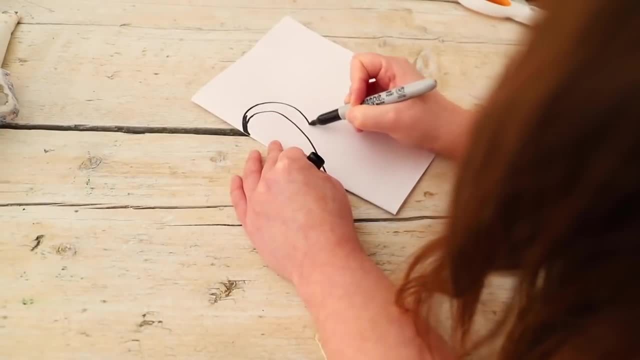 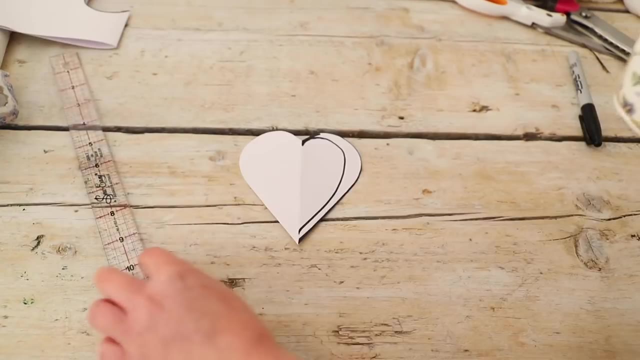 the paper in half. when you cut it, you'll get this perfectly symmetrical heart, even if you may have not perfectly symmetrically drawn your heart. So just a little tip: fold the piece of paper in half. I also just use my cup just to test out the size, to make sure that it was big enough. 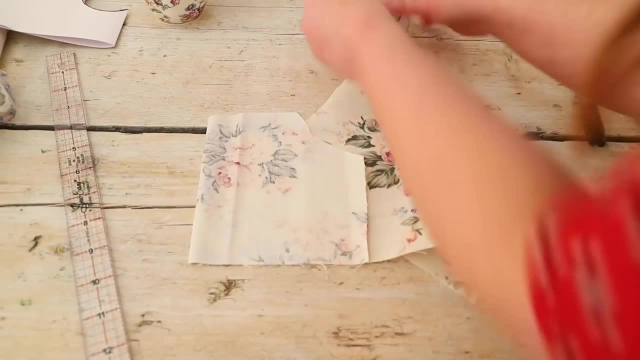 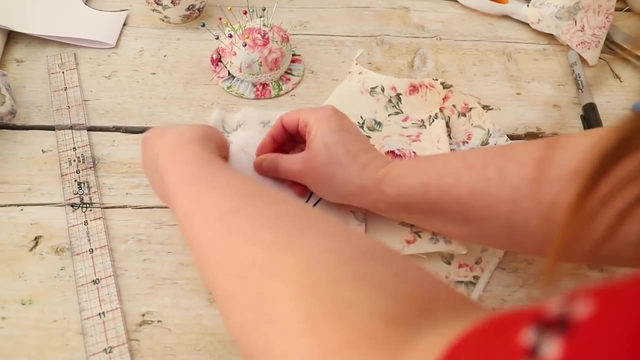 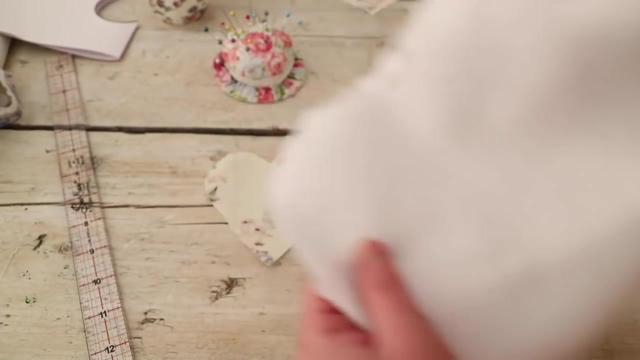 and that I had like the right size. To make this it's really simple, I folded over my scrap fabric and I placed my love heart on top, I pinned it and then I cut it out. I then used some fleece that I had lying around, and I also used that and cut it into the shape of a love heart. I then sandwiched. 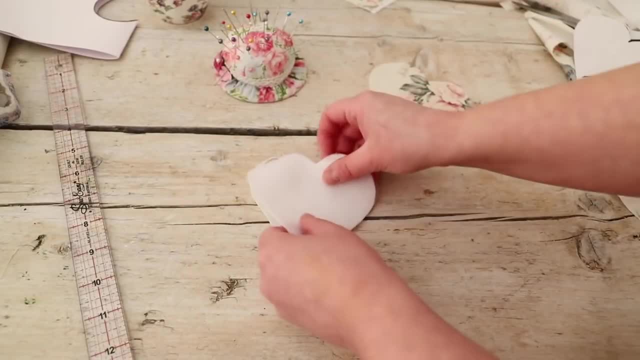 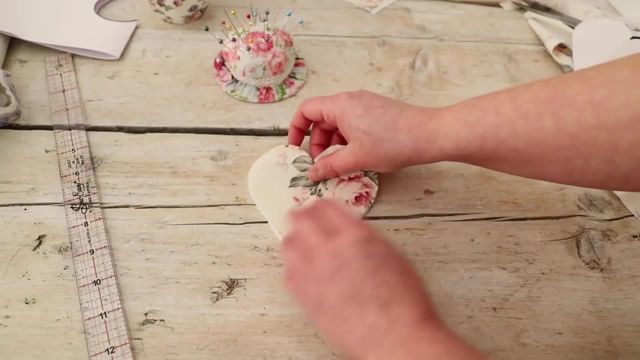 it all together. So I put the pattern piece facing down, I sandwiched on the felt and then I popped the top piece on and I'm going to simply stitch all the way around and then I'm going to use my pinking shears to trim the raw edge. This is so simple and so beginner friendly. You could. 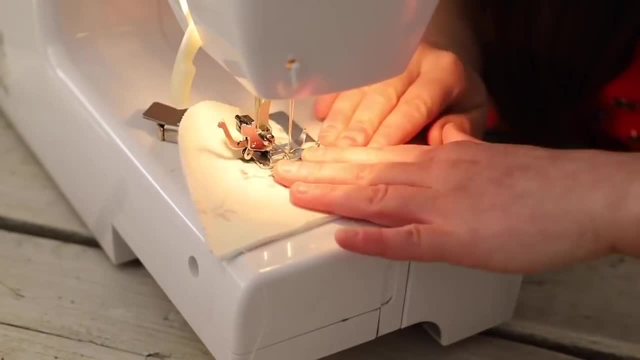 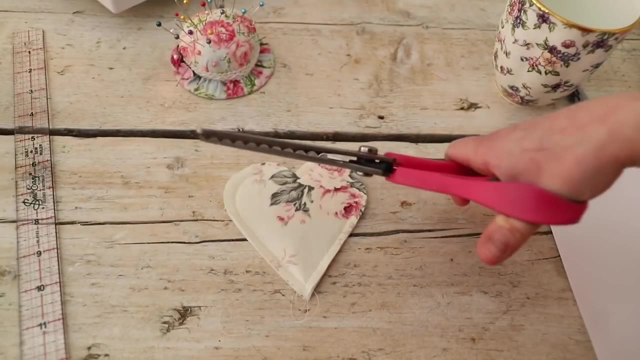 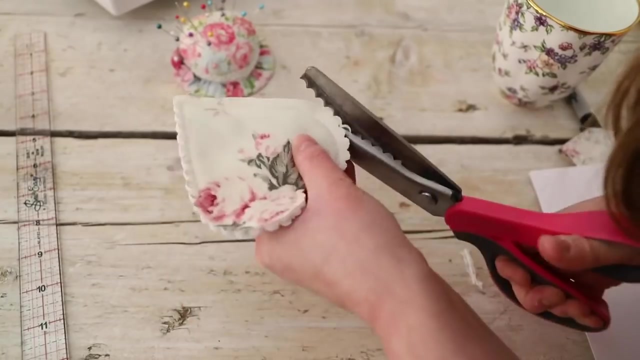 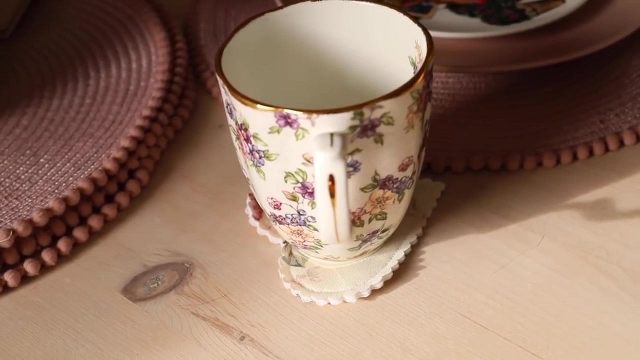 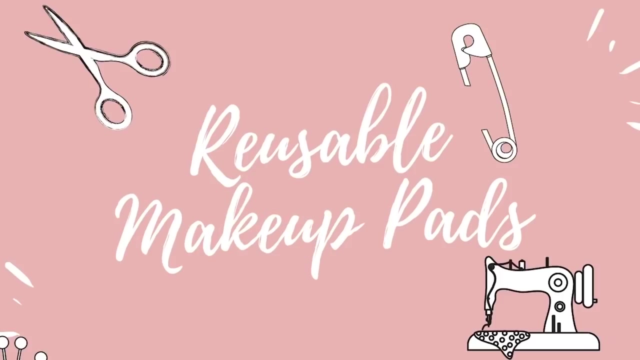 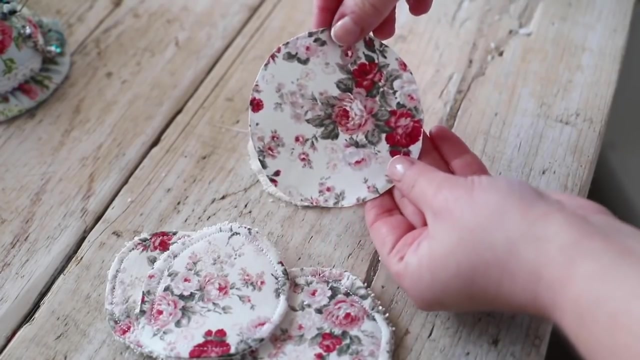 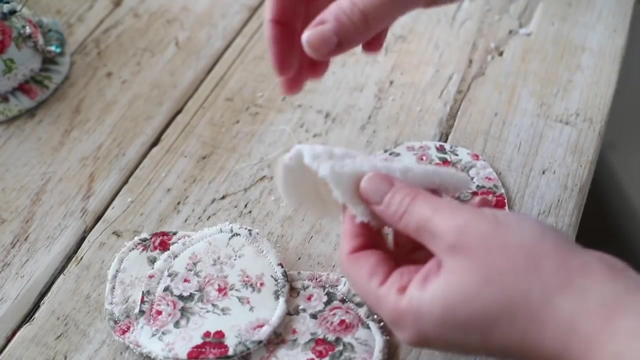 probably hand sew this, so if you've never actually sewn before, these will be really fun to make. It's so easy to make your own cotton pads. You don't have to use the disposable ones. So I actually use the end of a cup for the circle template for this. So I cut out two pieces of fabric. One is an. 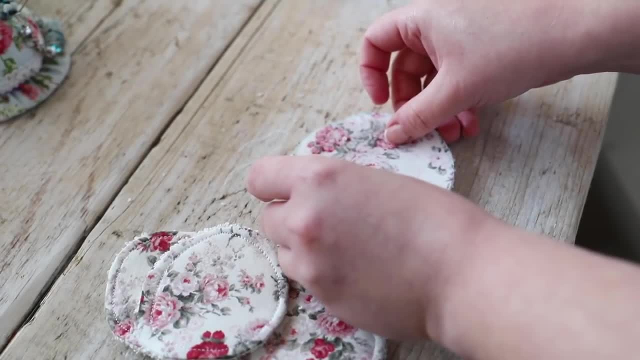 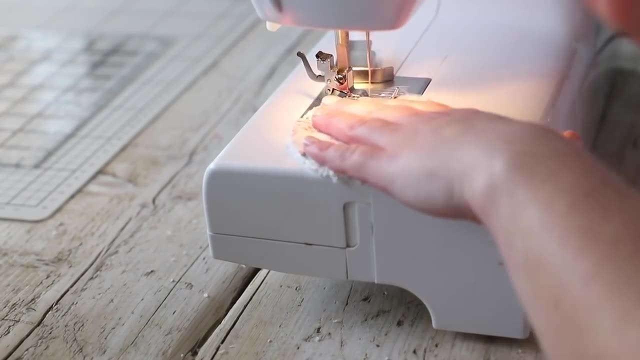 old piece of towel and the other is just a piece of cotton that I have. I'm placing them together with the right sides facing in. I'm going to use a piece of cotton that I have and I'm going to stitch all the way around, but I'm going to leave a gap so I can turn them right way out Once I have. 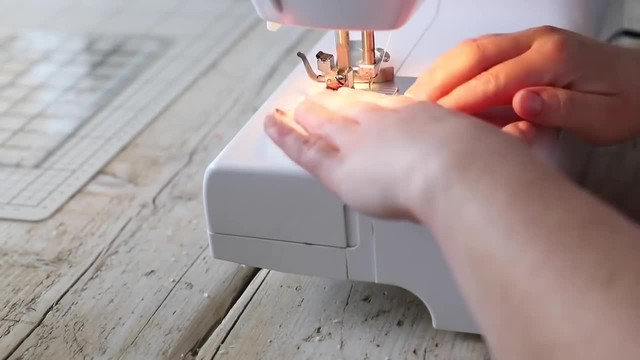 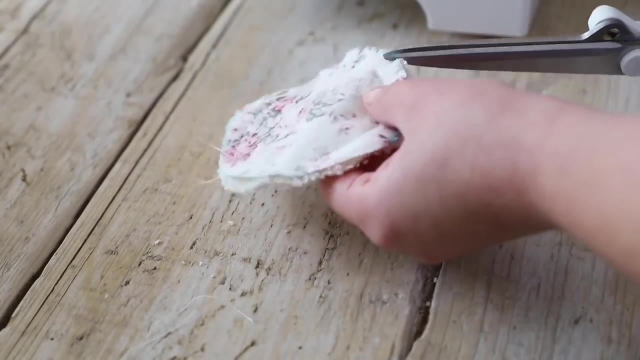 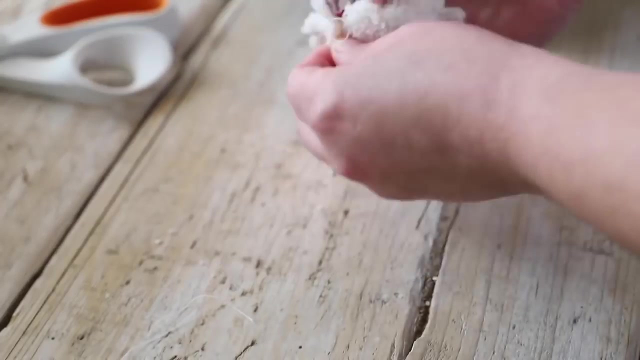 turned it right way out, I will clip the curves. This just makes it like not as square, if that makes sense. It just keeps the circular shape, but you can customize this and make them bigger or smaller, depending on what you need. I'm going to turn the fabric right way out and then I'm going 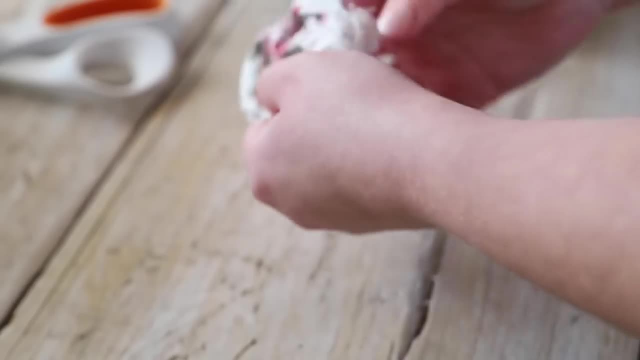 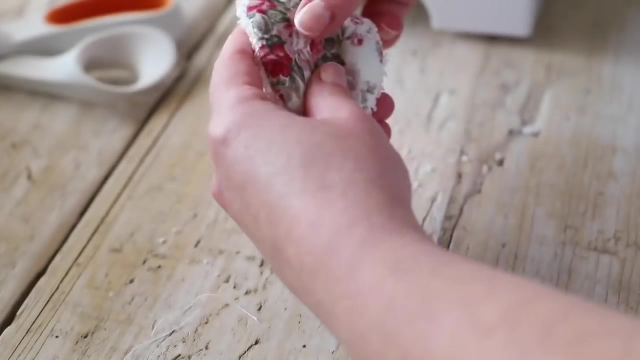 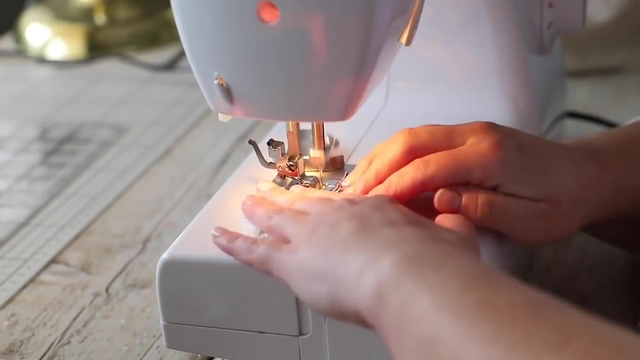 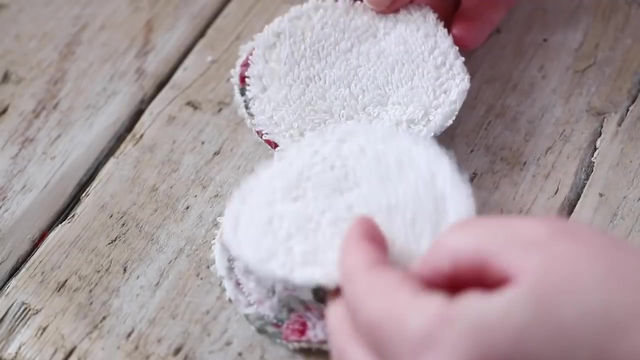 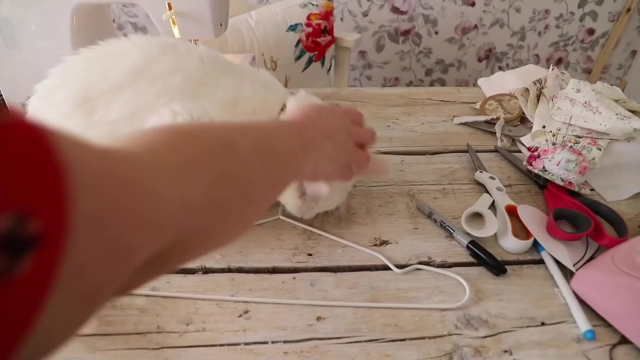 to do a top stitch and I'm going to fold in that opening and do a top stitch. So I'm going to do a top stitch and you have your very own makeup pad. So next up we have some fabric hangers I randomly had. 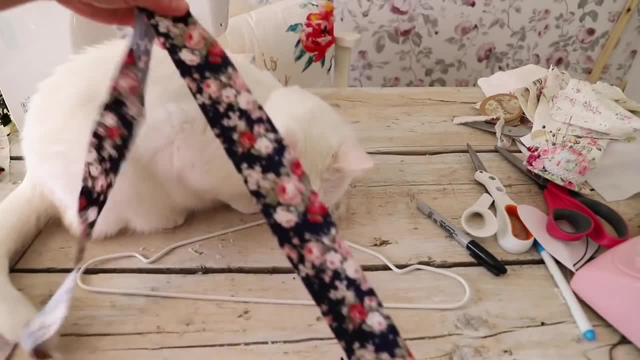 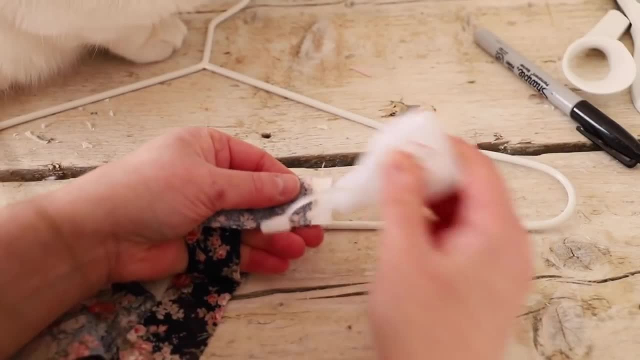 strips of fabric. I think this is because I was doing like a blanket and I ended up with longer strips of scrap, So if you are a blanket maker, this might be a good one for you. I actually ran out of glue gun sticks, which is why I'm just using some cheap sticky glue, So I glued the top and I 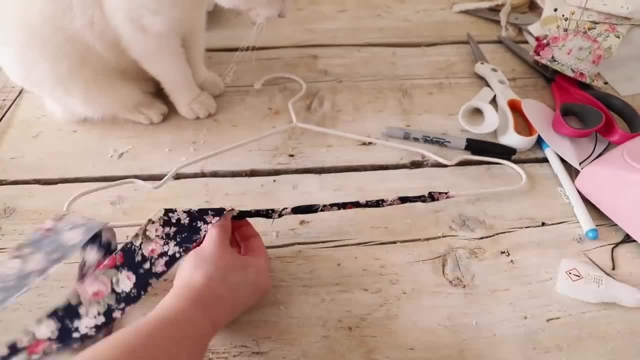 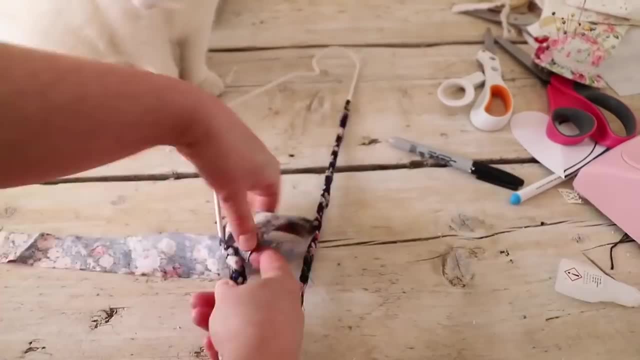 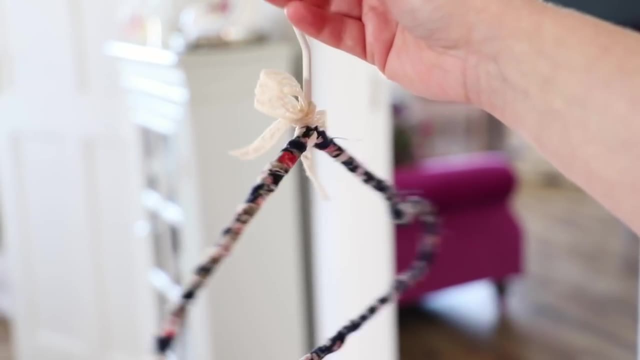 simply wrapped fabric around the whole hanger- If you have like a plastic hanger, you could probably do this as well- And once I got to the end, I simply glued it in place and that was it. This is so simple and you can layer up your fabric strips, So like. I took two strips to do this, but you could. 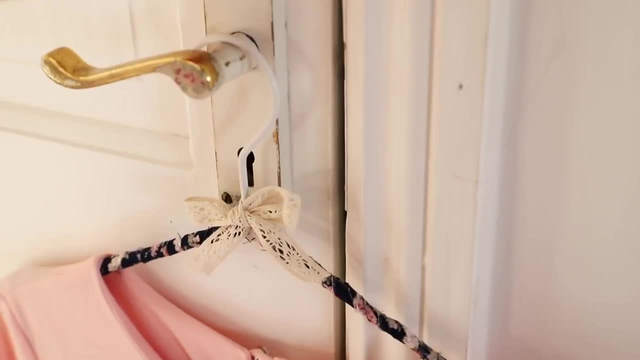 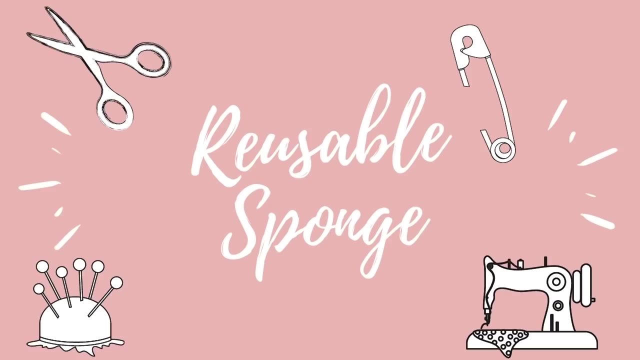 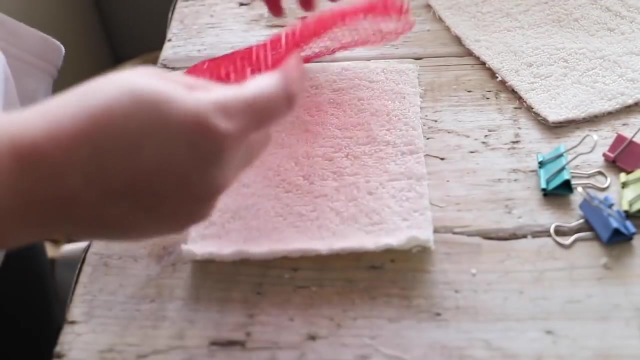 mix and match with loads and also the raw edge kind of gives it a little bit of character. Hands up, who doesn't have a dishwasher and uses sponges to clean the dishes Me, So these are really easy to make. I'm using more of the recycled towel fabric and I'm just 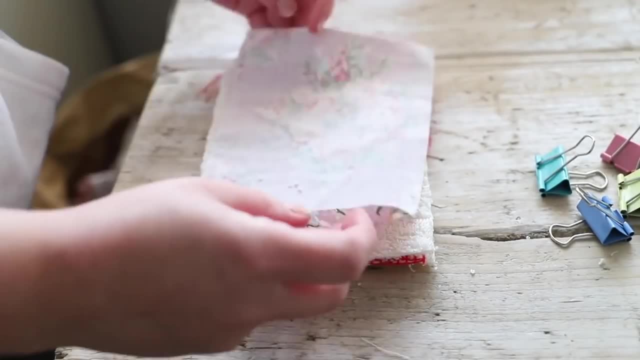 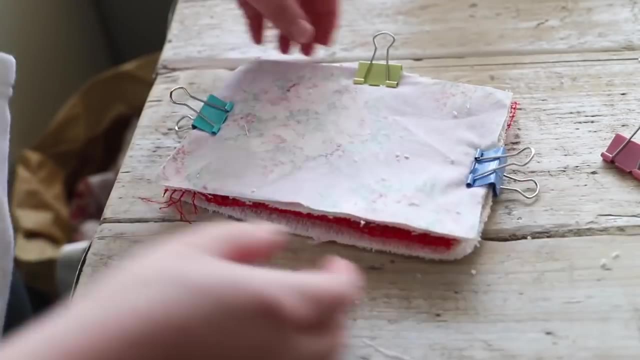 sandwiching it around. So I'm going to do a little bit of this and then I'm going to do a little bit of, together with a piece of. actually, that plastic was from my fire logs. It came in this little package, So I just recycled it and I'm using that as the lining of my sponge, So I've sandwiched it. 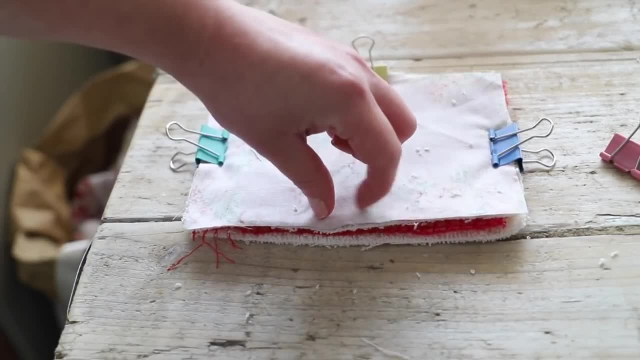 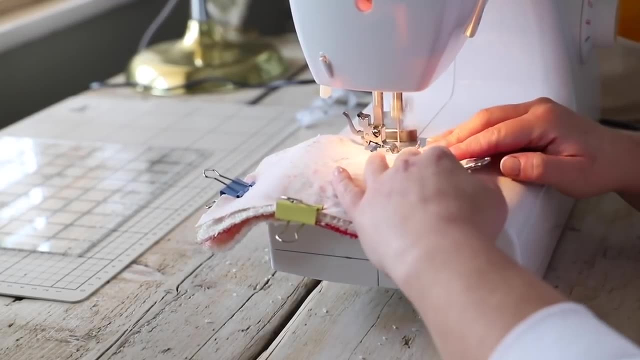 all together, as you can see, with the right side facing down of the cotton fabric, Just like the makeup pad. I am stitching all the way around, but I'm leaving an opening. Don't forget to do a reverse stitch at the start and the end of your stitching. Once all of this is stitched, I'm going to 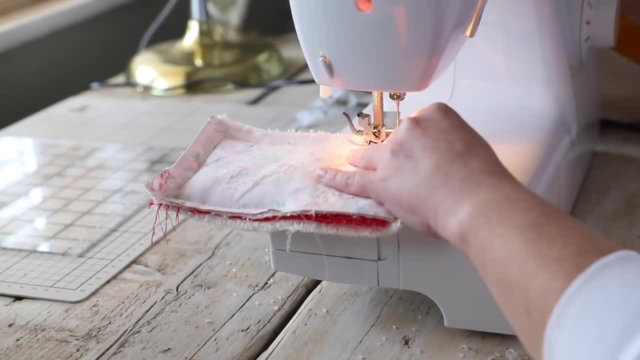 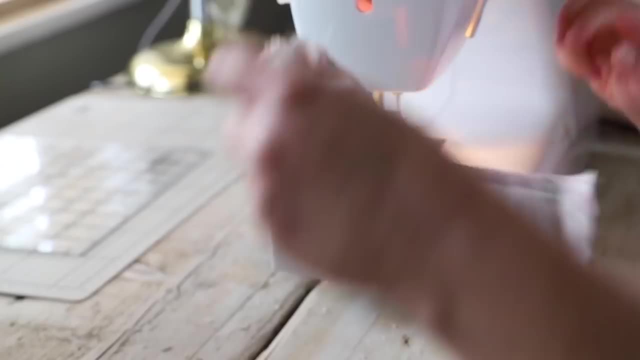 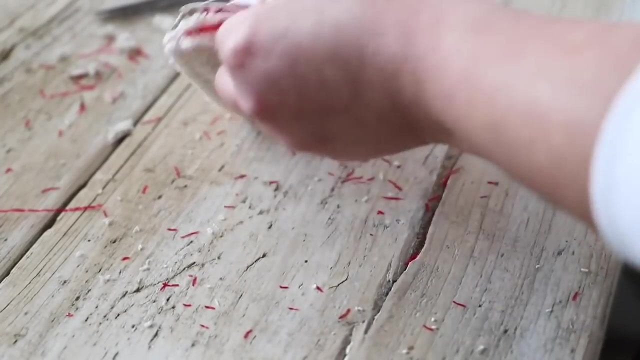 pull it right way out again. Same as the makeup pads, but it's just a different shape and more fabric. Also, just before you turn it out, just clip the corners as well and then turn it right way out, and then I did a top stitch on this as well, and then you have your very own dishcloth- Also this: 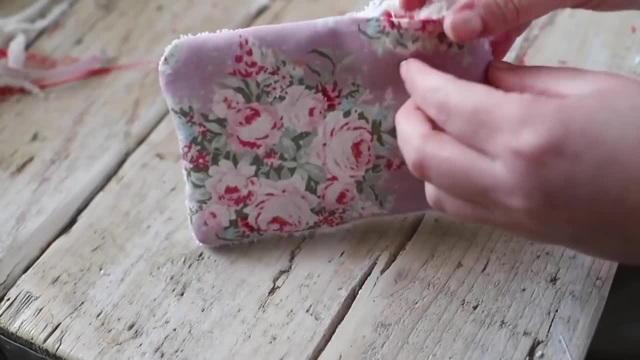 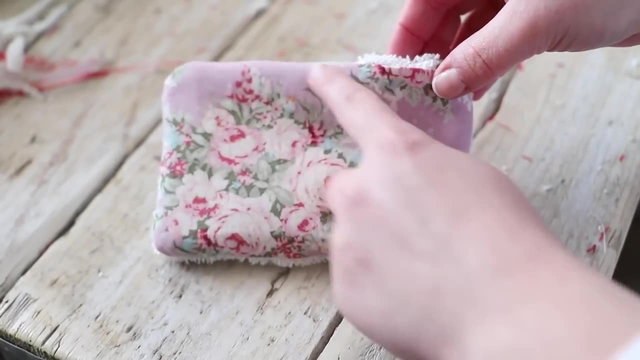 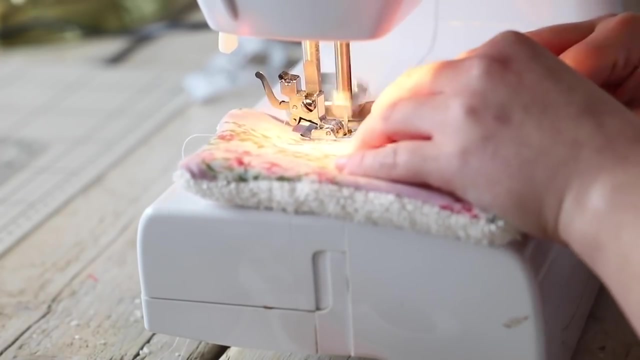 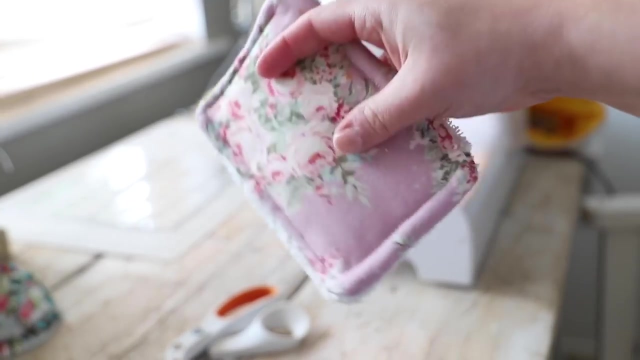 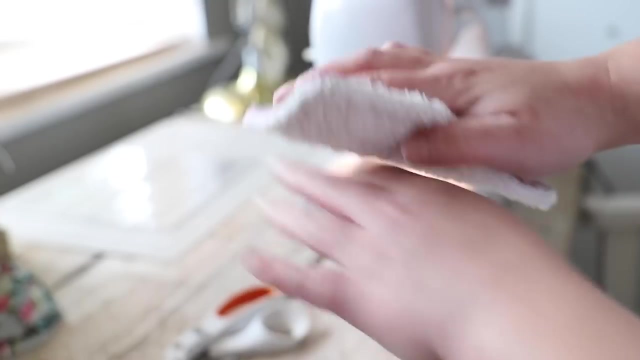 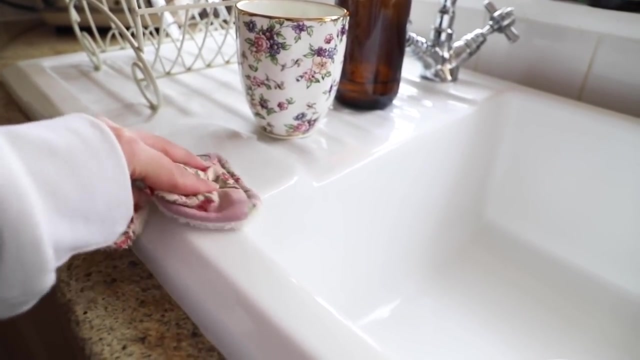 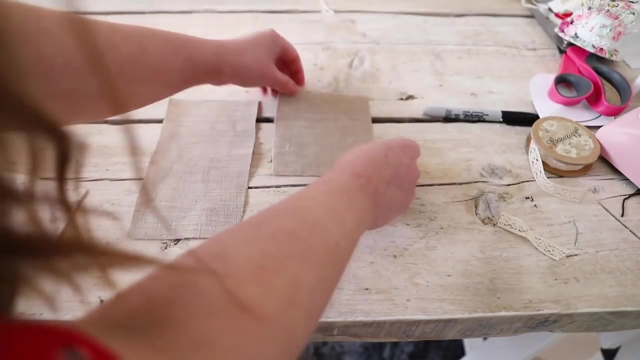 could be. maybe if you use like face wash or you need something like more exfoliant, you could probably use it on your face as well. But I'm using this thicker pad for doing the dishes Next up. I'm making a little pouch, So I'm actually doing a catnip pouch for the cats and just to thank. 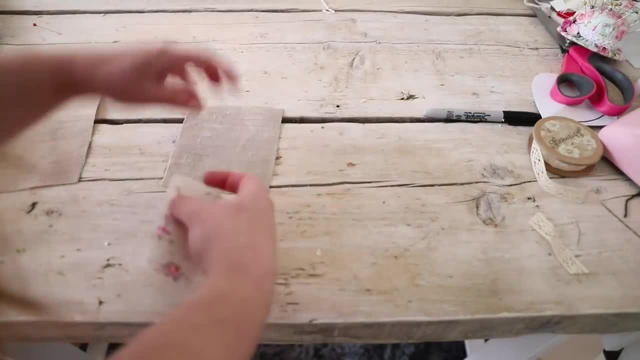 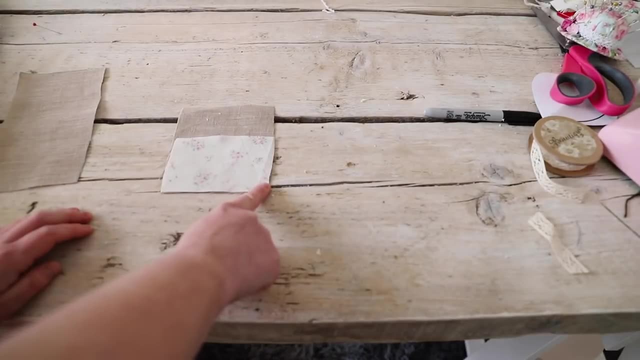 them because I'm off work at the moment and they're probably sick of seeing me. You can also make up your own measurements for this, So I simply have two sides, but on the front side I'm using two pieces of fabric. So, as you can see, I joined them together and I just ironed my seam. 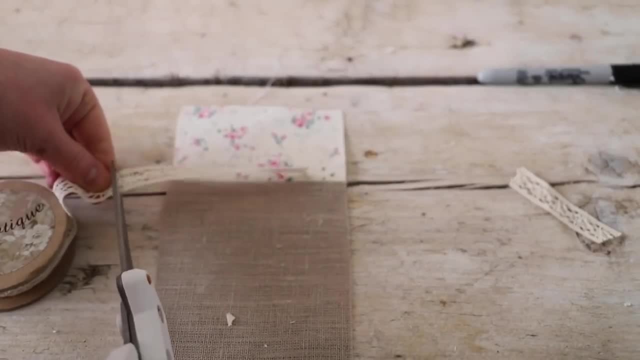 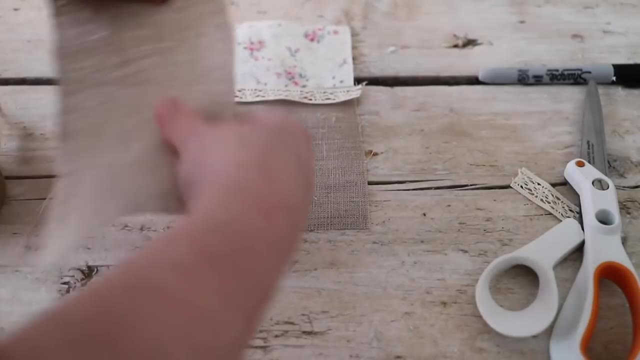 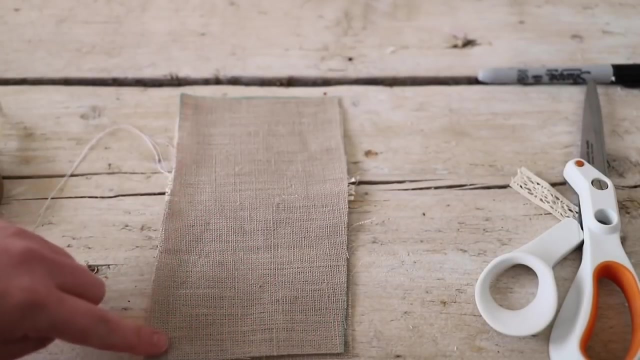 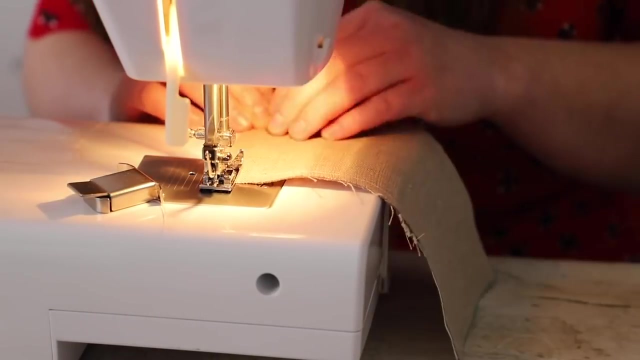 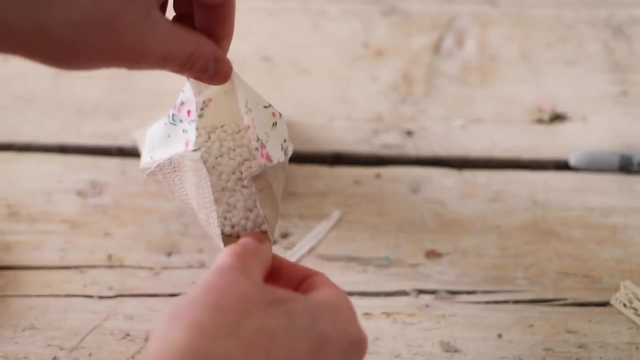 So that gives me the front panel. I added a little bit of trim and then I put the two right sides of fabric together. I stitched it all the way around and I left an opening at the top. I got these all. they're like little squishy balls. I actually took them from. 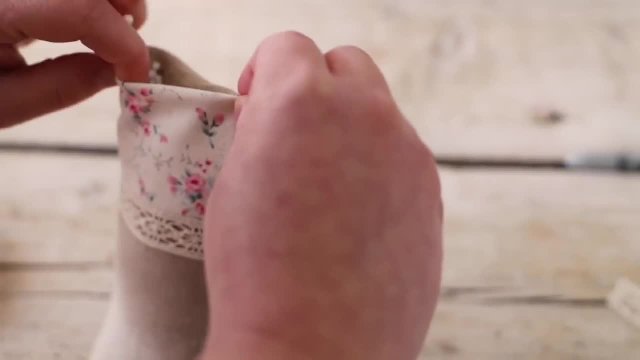 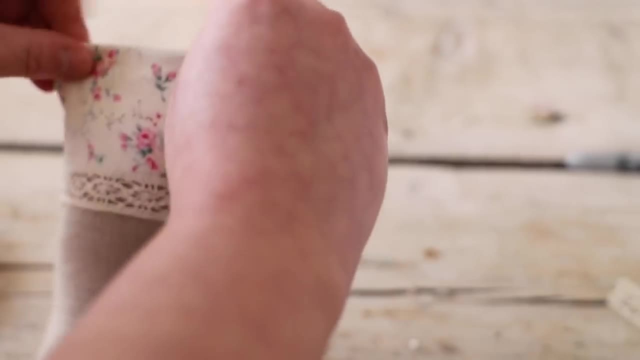 an older Shore, L 사람들이. They're like little squishy balls. I actually took them from an old um toy that the cats had and that they had absolutely wrecked. so I recycled them and popped them in this and I just put some fresh catnip inside. I folded the top. now, if you are making, 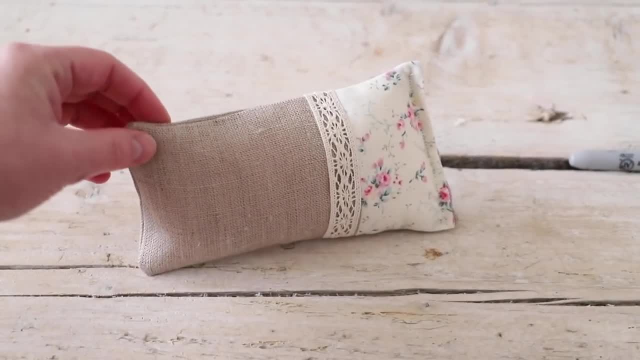 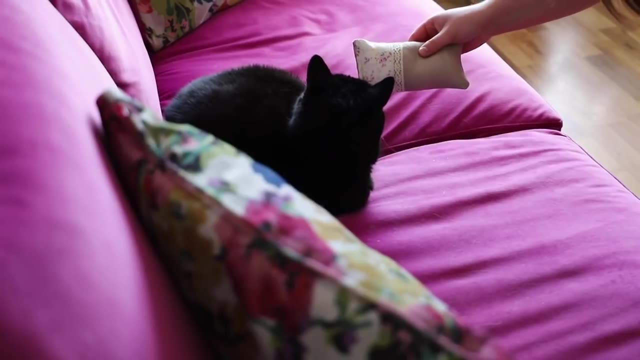 a lavender sachet. you could hand stitch it, but because I need this to be durable, I machine stitched it because, as you will see, these cats are ruthless when it comes to the catnip pouch. I'm also going to pop in an old clip of when I made a cat collar, because it's a great way of 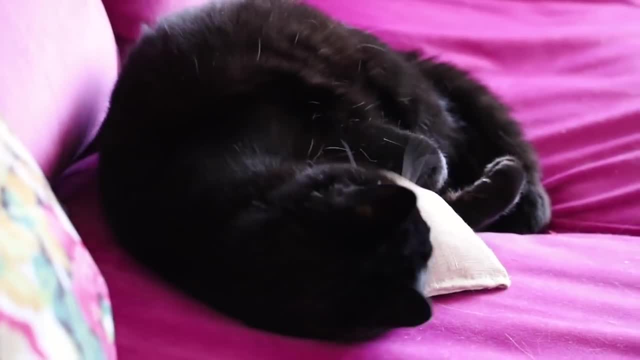 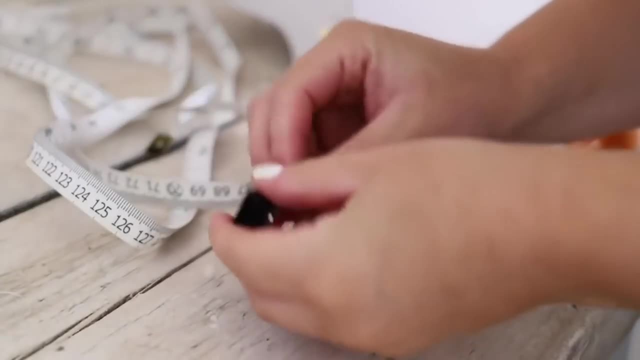 using scraps. so some of you may have already seen the next project, but I just wanted to pop it in for anybody who hadn't seen it. so I'm going to make some cat collars. we are going to be using an old collar as a template and we are going to make a brand new collar for Blondie. I'm going to 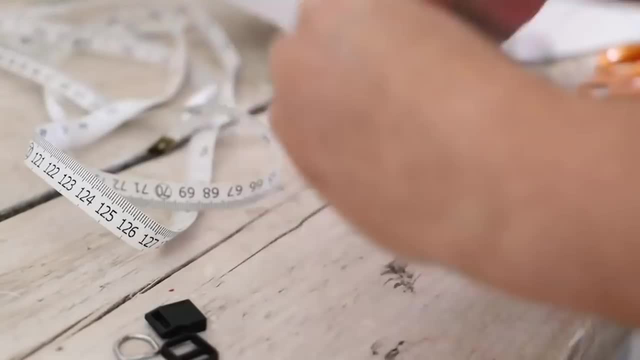 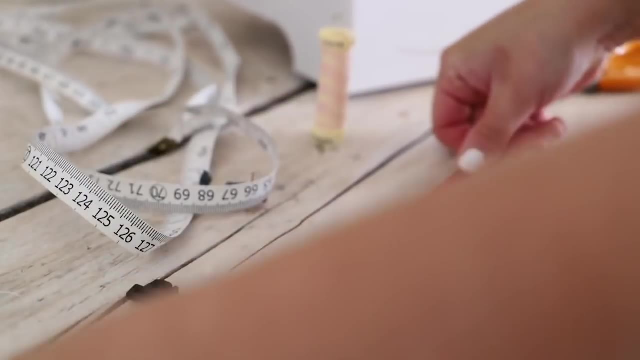 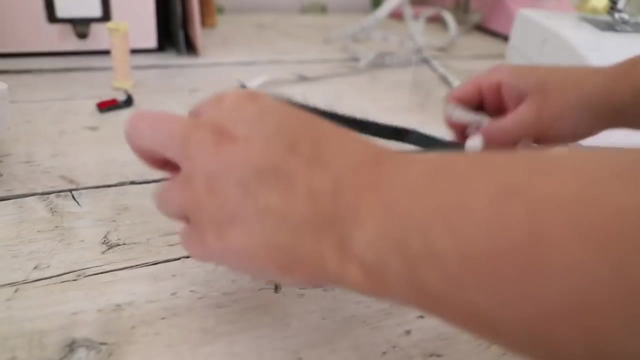 use some scrap fabric for this, and this is really simple to do. the first thing I'm going to do is dismantle the old collar and take all of the pieces off. so this old collar has safety clips and I'm just going to recycle them and I'm going to use the old piece of fabric as a template for the new one. so I'm just measuring. 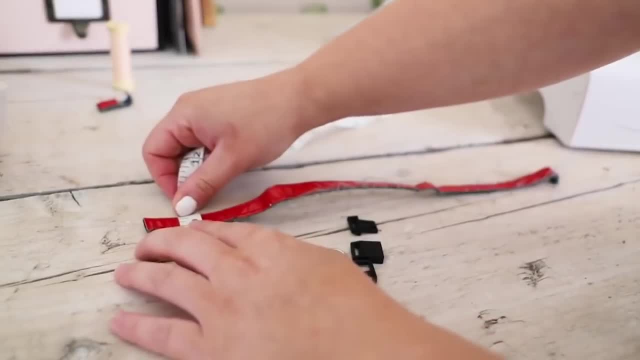 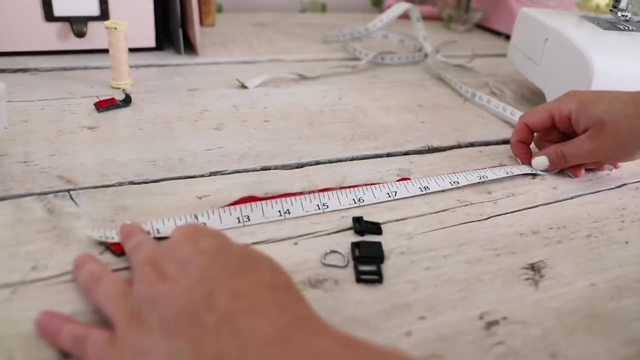 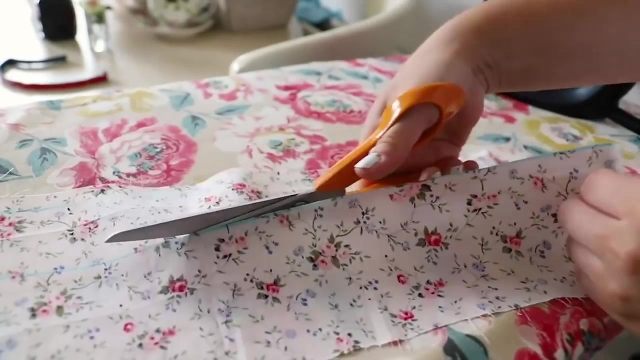 across and down and I'm going to add extra fabric. I will put the measurements in the description box if you want to follow along, because I think most of these and cat collars they're kind of the same size, so I will pop the measurements in the description box. I just use my sewing marker. 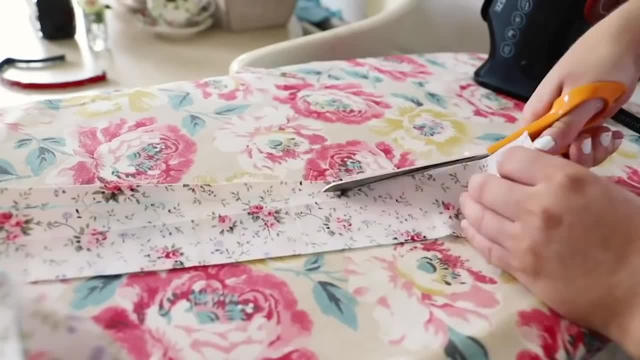 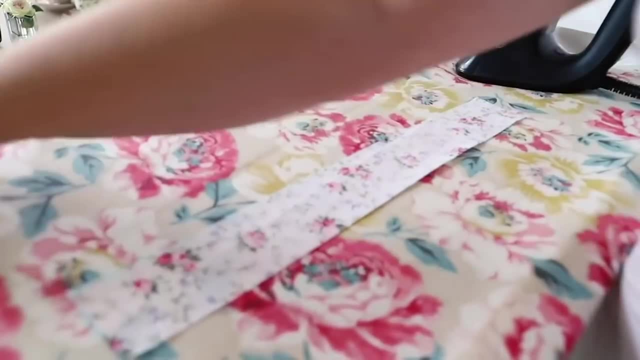 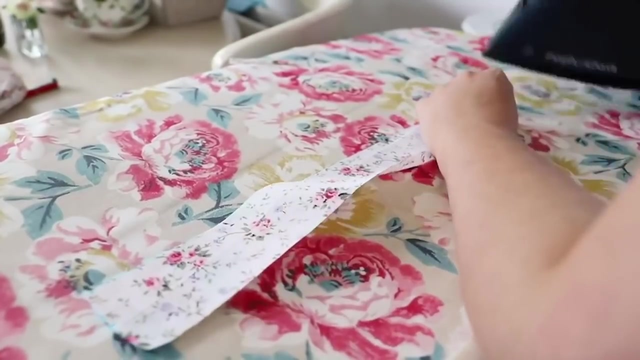 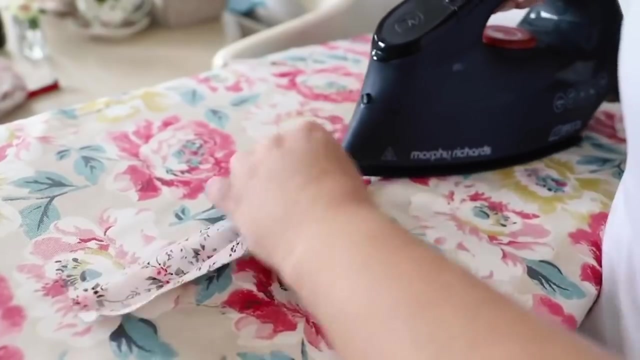 and so once you apply water, this will dissolve. so I just measured on the measurements to the fabric directly and I cut it out. so for this, I simply found the center of my fabric and I folded both sides inward- which I hope will make sense when you watch what I do- and then I folded it in half again and this is going to be. 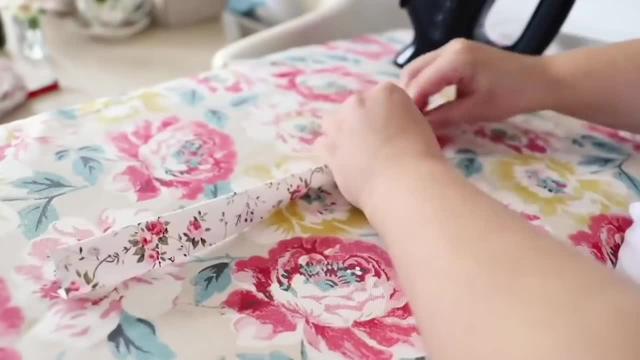 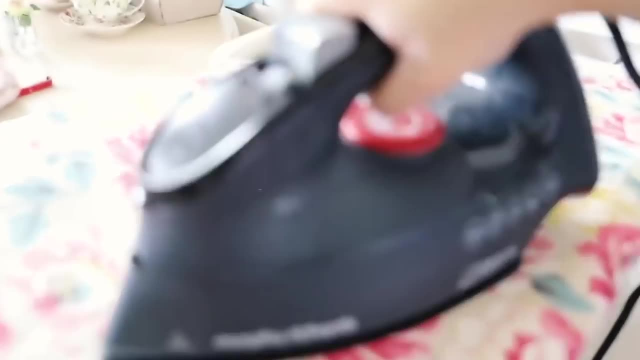 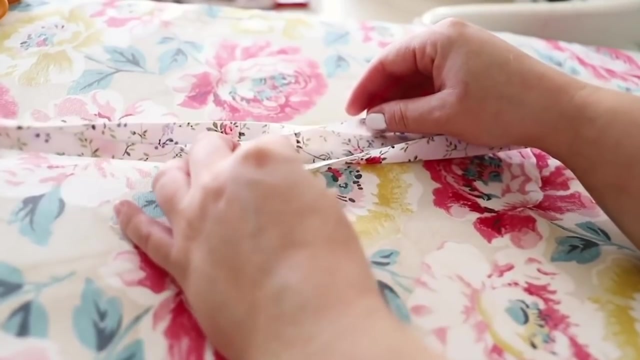 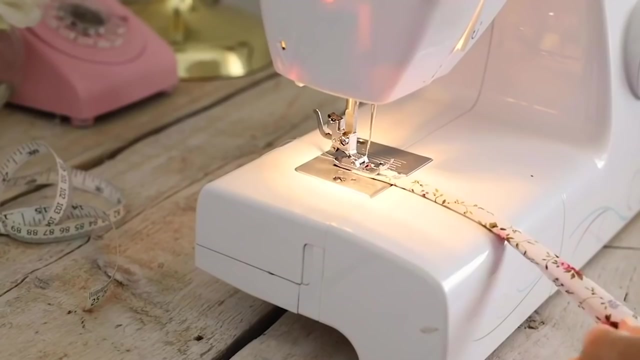 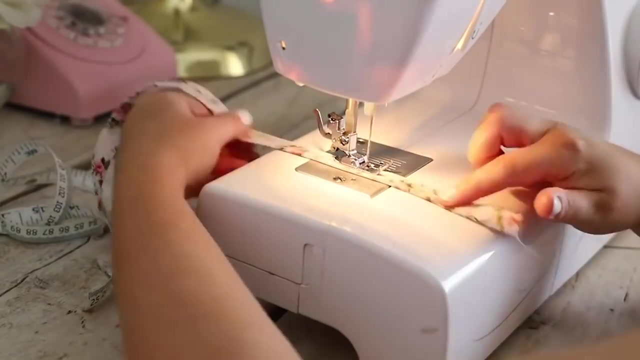 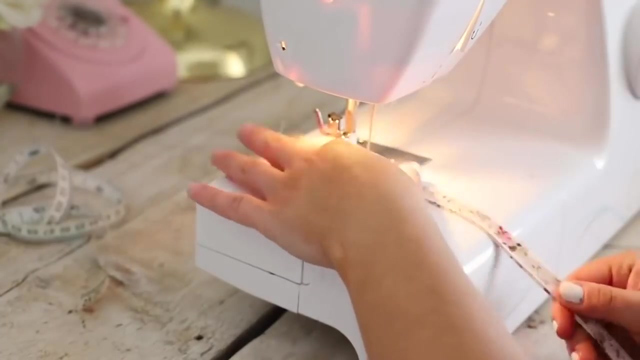 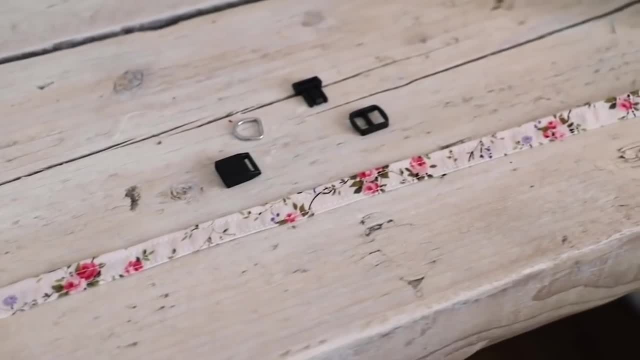 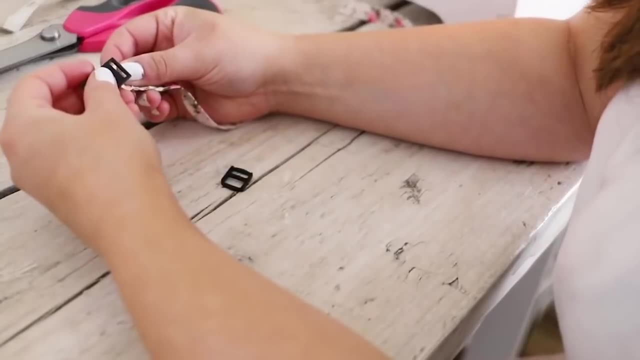 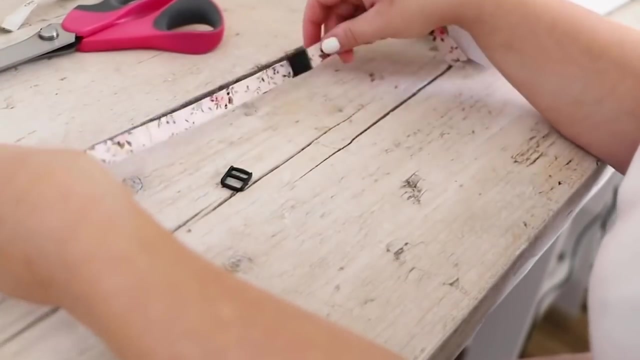 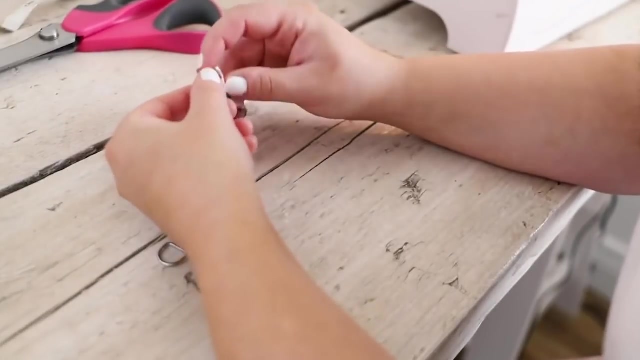 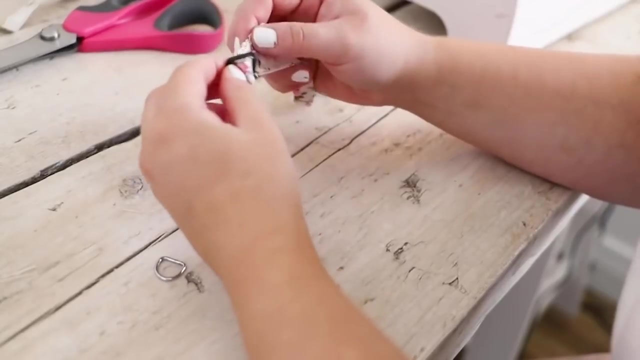 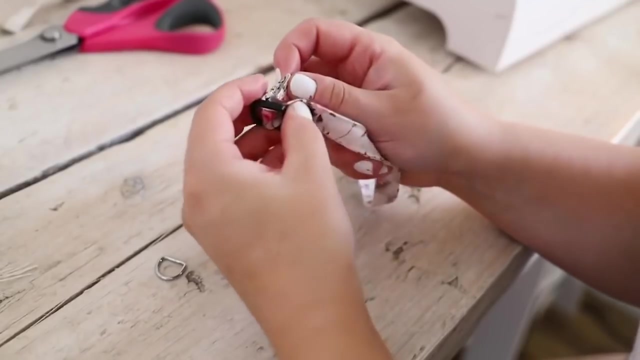 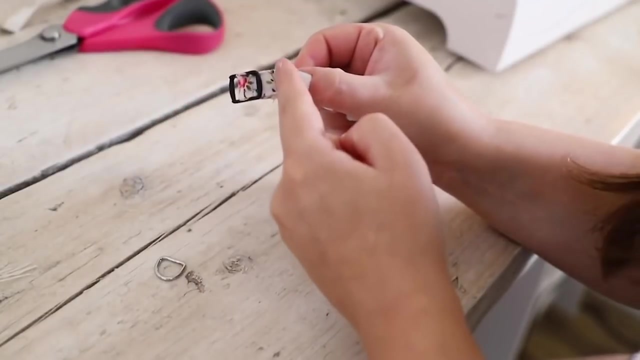 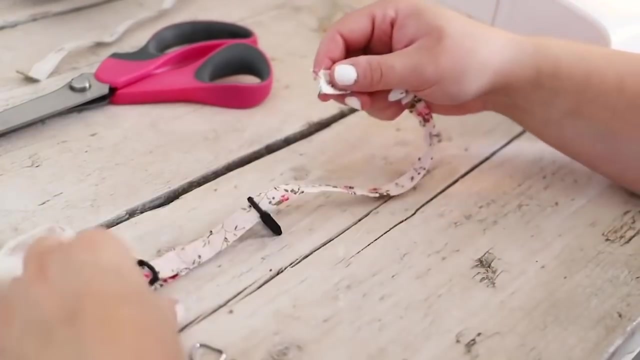 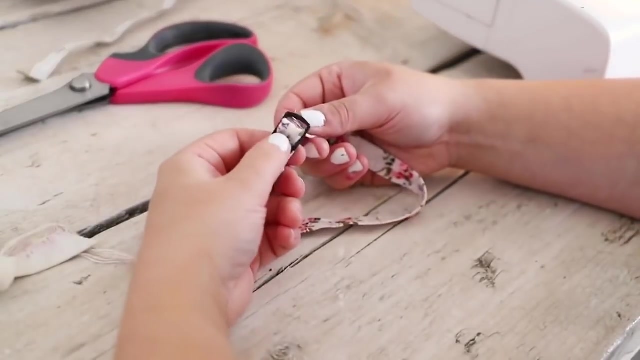 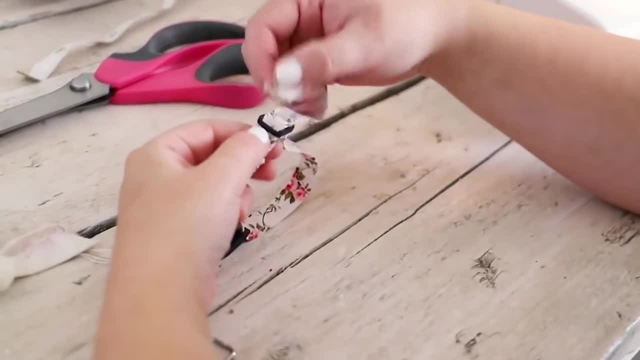 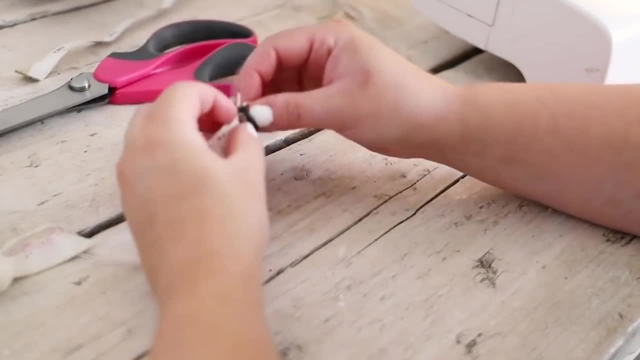 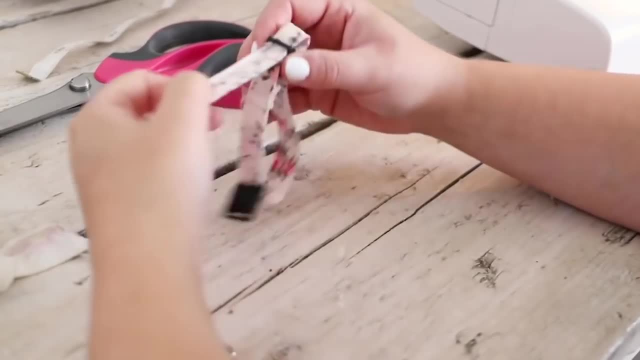 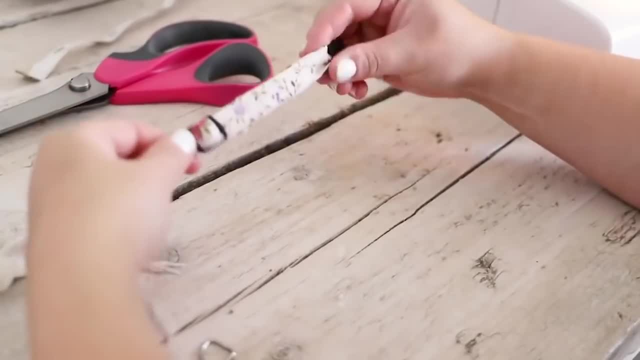 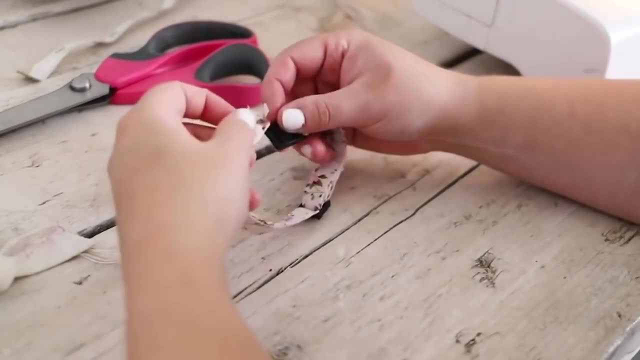 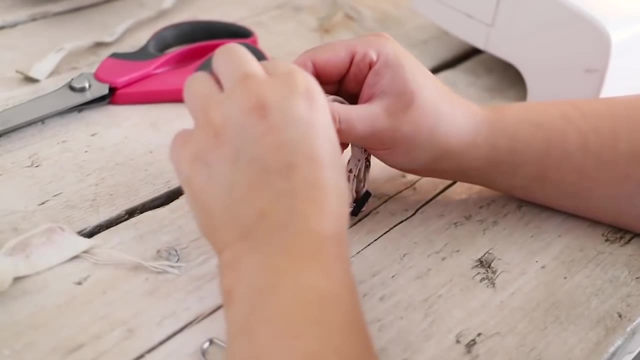 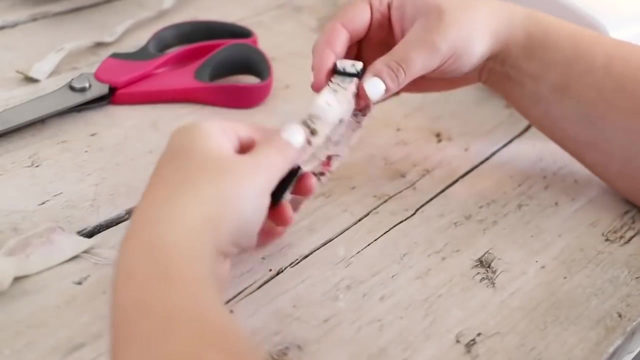 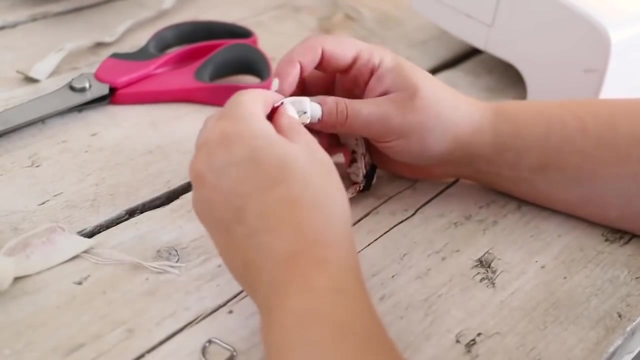 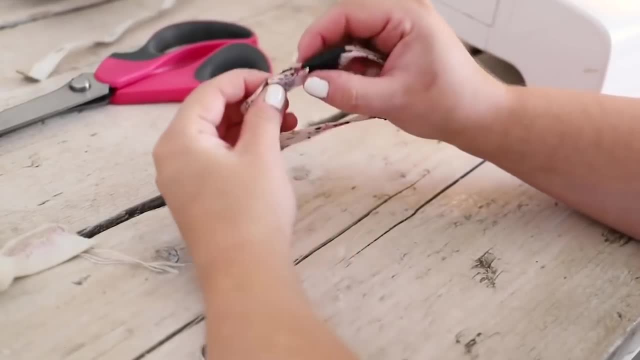 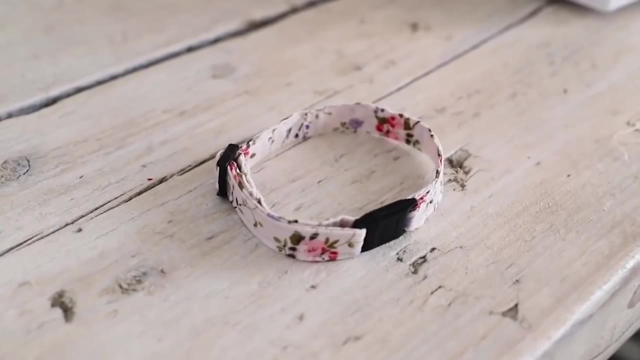 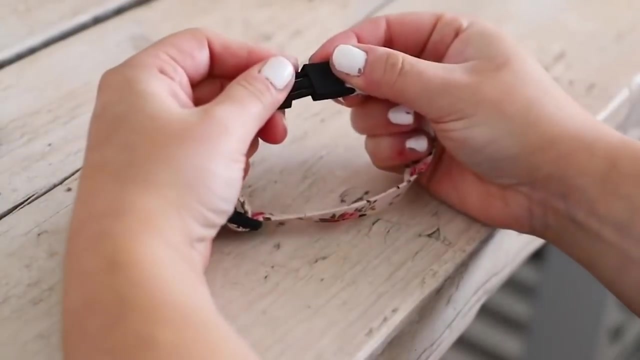 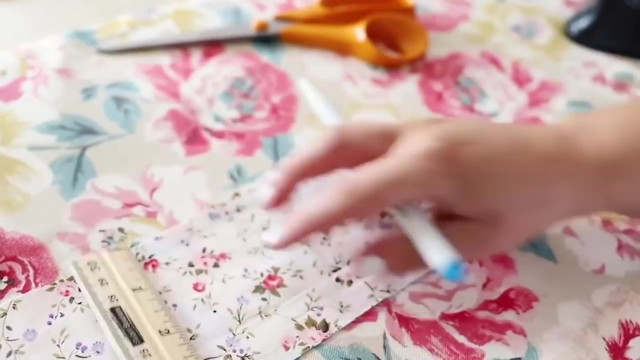 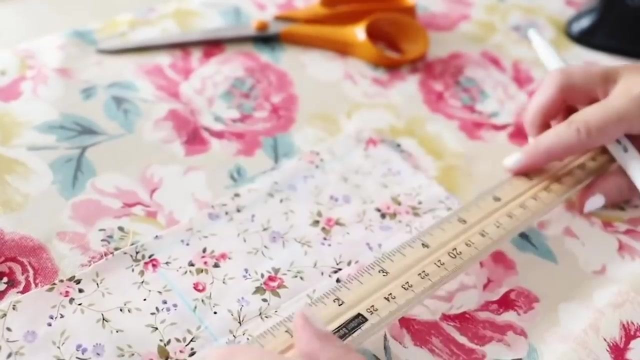 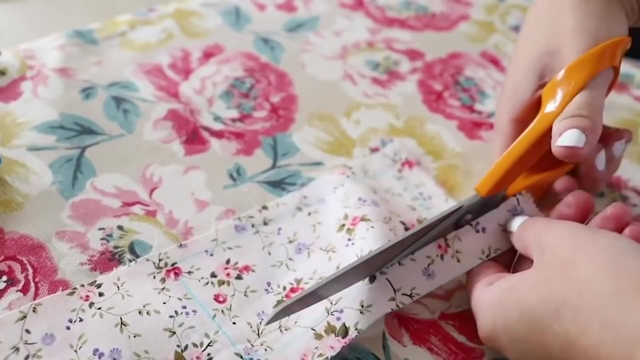 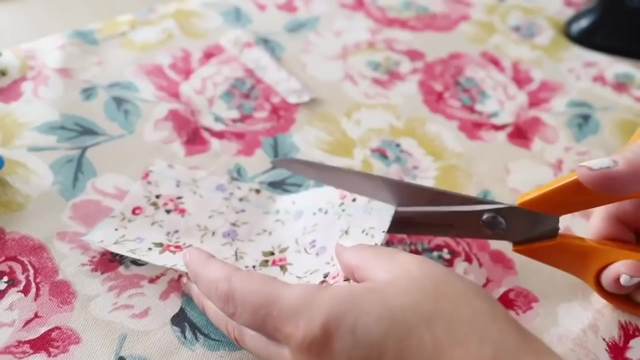 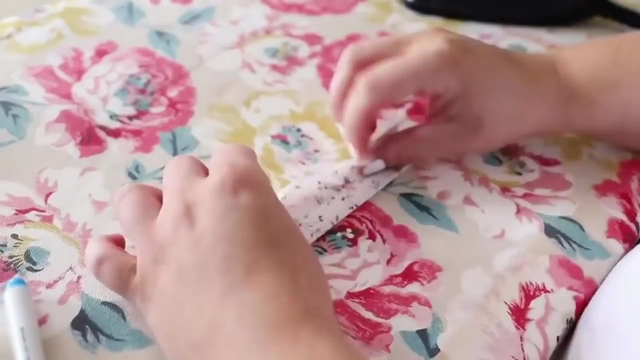 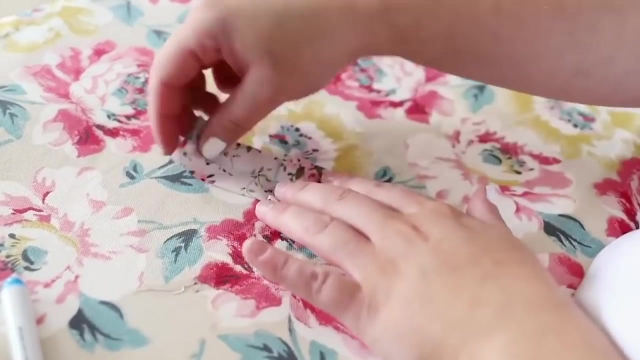 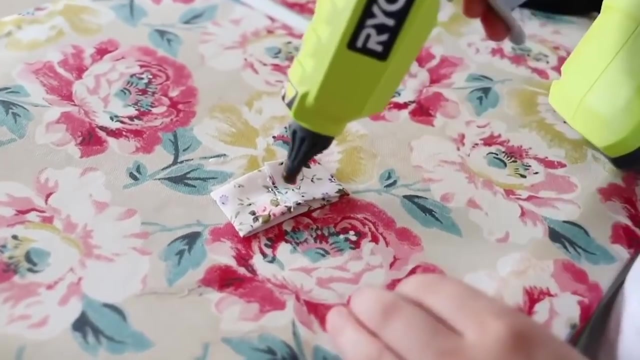 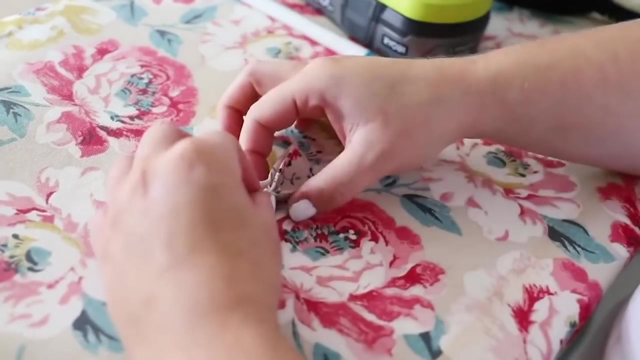 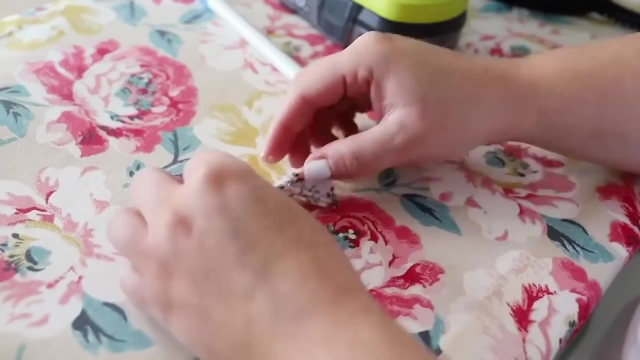 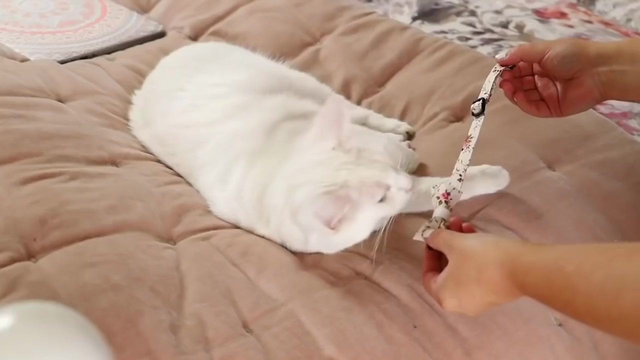 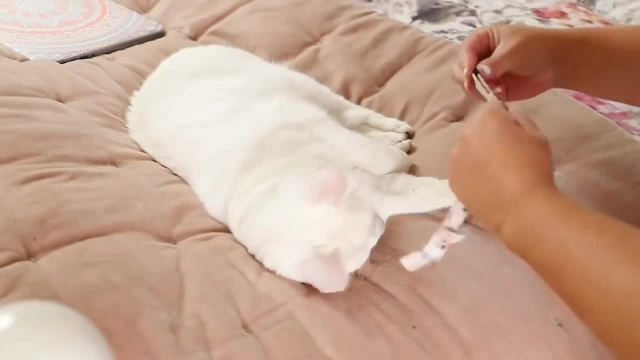 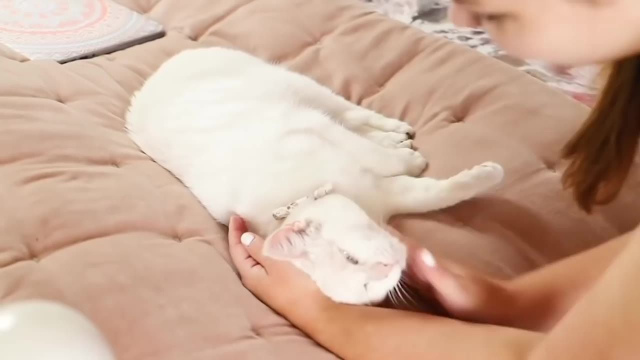 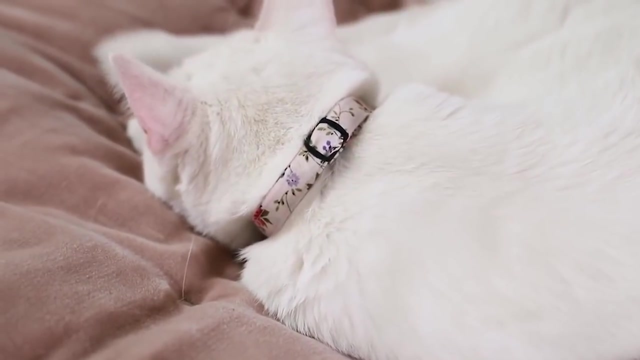 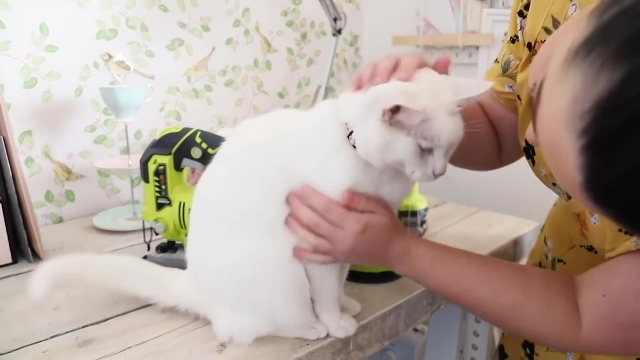 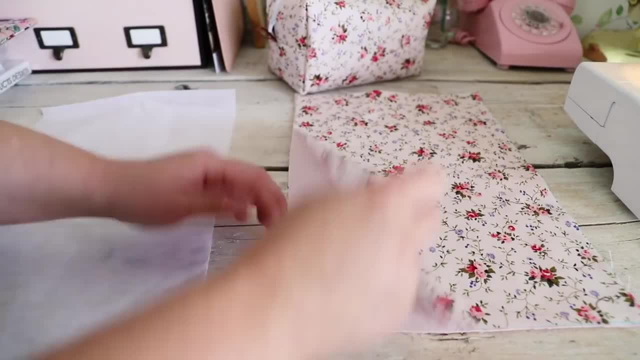 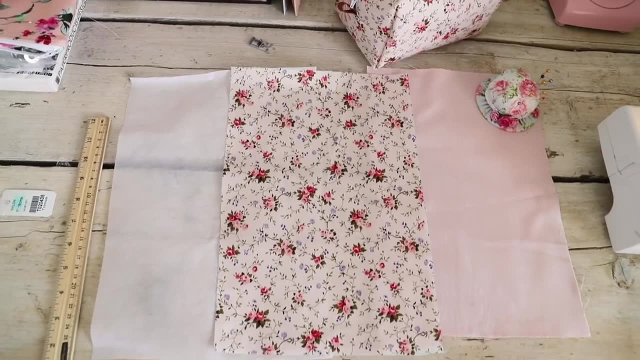 going to be making two pouches. This is the first one, which is going to be a boxy pencil case style. We have three pieces of fabric for this. We've got a front piece, a lining piece and I have some iron-on interfacing. I will also. 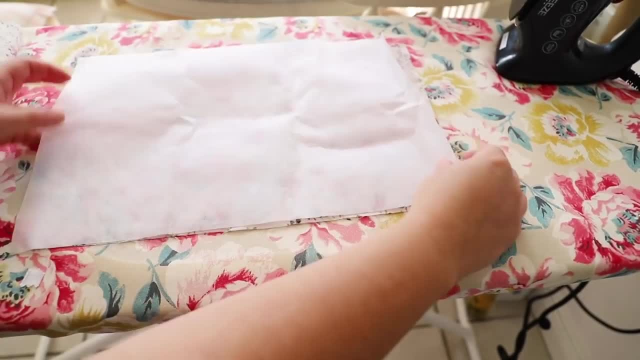 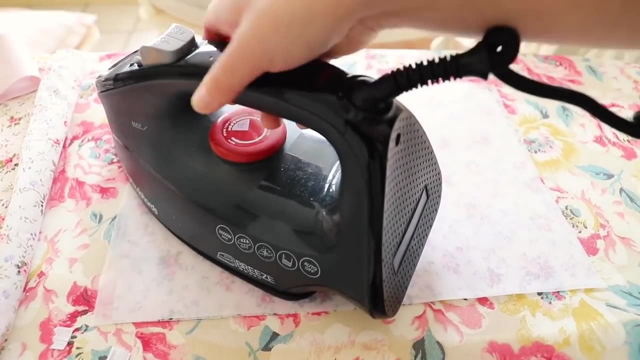 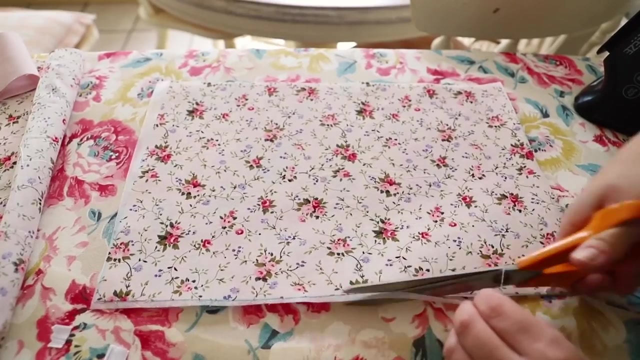 leave the measurements in the description box. The first thing I'm doing is ironing on some iron-on interfacing. This basically stiffens the fabric. so when you're making pencil cases, pouches, makeup pouches, you want it to have some structure and hold its shape. Same if you're making handbags, You 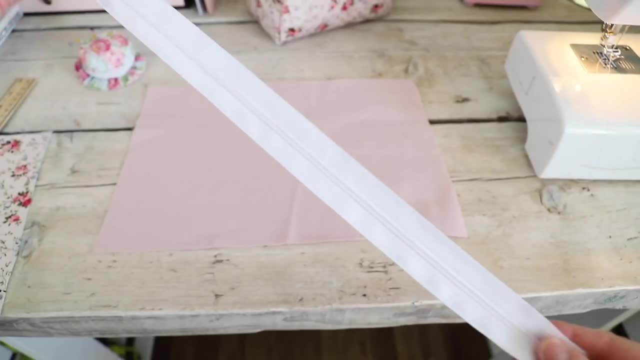 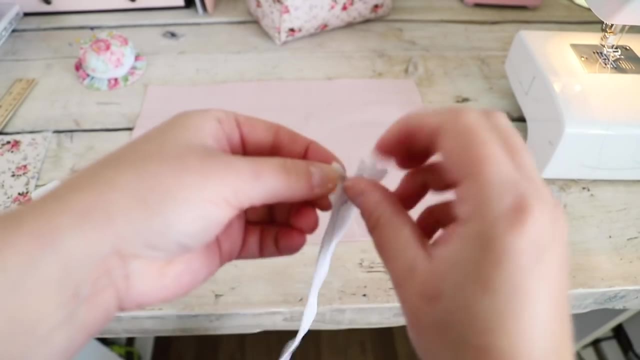 simply just iron this on and that is it. I'm then just adding my zipper. So I've got a 13 inch zipper for this project, but I'll leave all the details in the description box. You can also customize this to suit whatever size you want. I am. 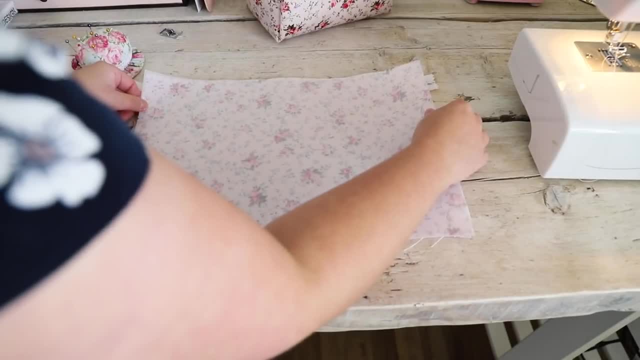 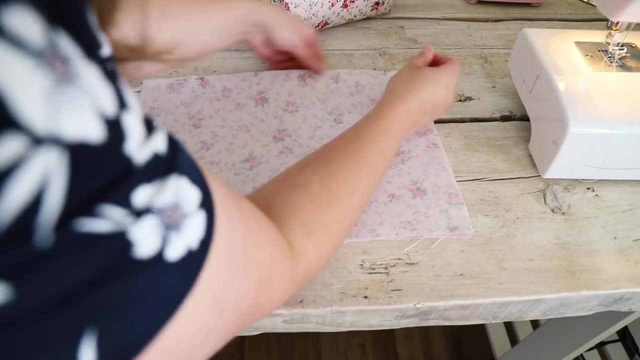 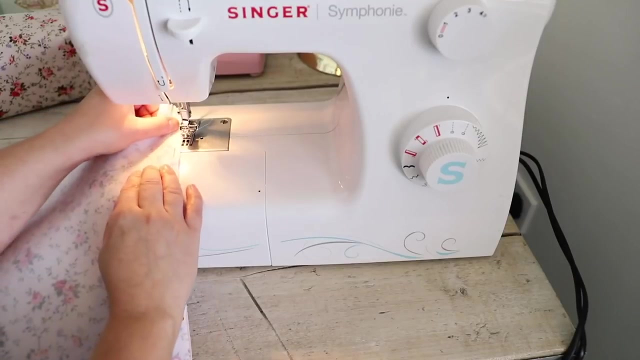 placing the closed zipper facing up against the lining fabric. I'm then placing the patterned fabric face down and I'm pinning it in place. I have seen people use these really cool clamps. Unfortunately, I couldn't get my hand on these clamps. I'm gonna have to order them online, but you can use them instead. 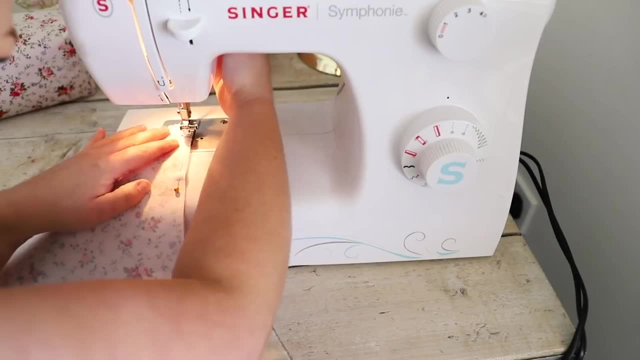 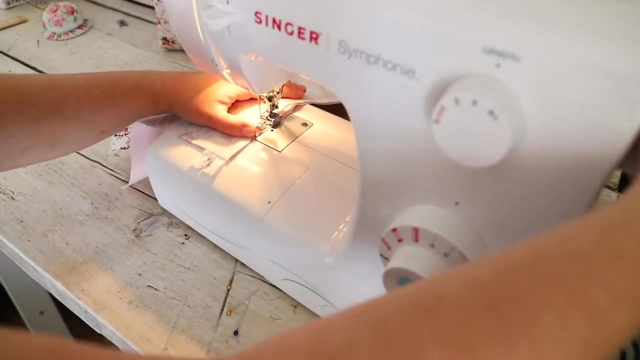 of pins. if it's easier When sewing you can use a zipper foot. You can pick up a zipper foot off Amazon really cheaply When you're sewing straight down, when you get to the bottom and you can feel the zipper with the needle still in. 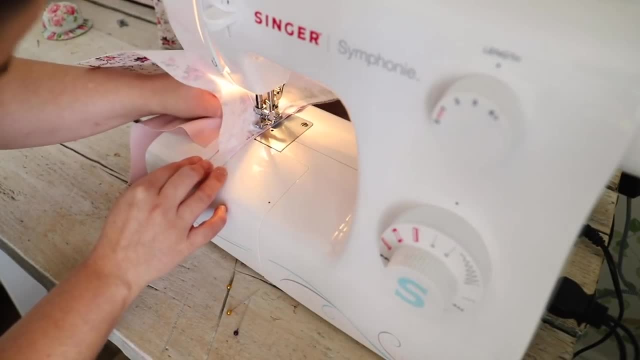 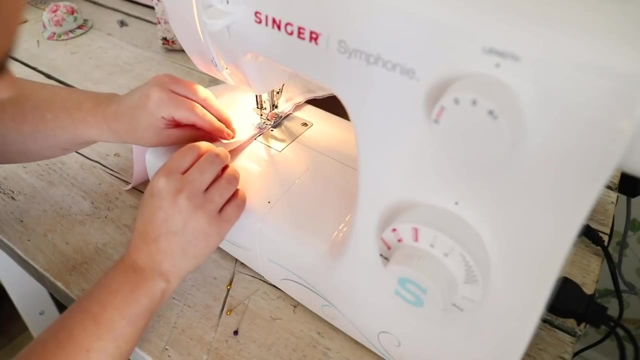 the fabric. you can just simply pull up the zipper. If you try and sew straight down, you're gonna get a wiggly line. You will see people just doing this. They'll be pausing, they'll be pushing the zipper, oh, and then they will be sewing back down. I hope that makes sense, but it's just so. 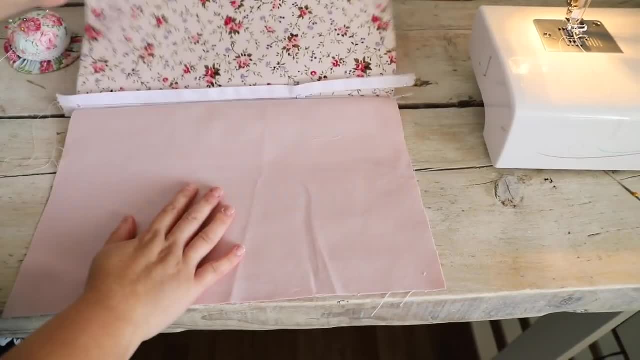 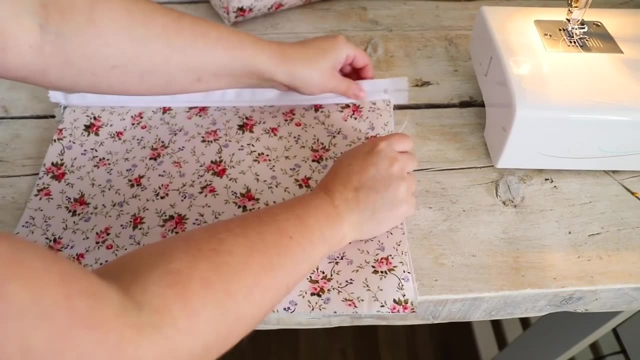 you don't get a wobbly line when you're sewing. So once you are happy and you are all sewed, you are going to iron this flat. I like to use the iron. It just gives it a nice professional finish and it just makes it neater. Once I have it ironed, I press it in. Once I have it ironed, I press it in, And once I have it ironed, I press it in When I put the zipper on and I sew it in. it should be easy and simple. You just need to mark it as you're sewing and I just put it in. 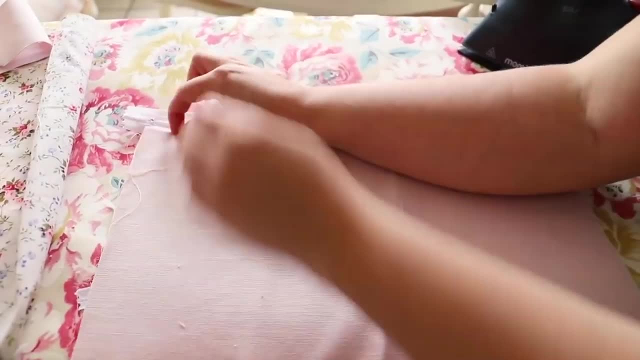 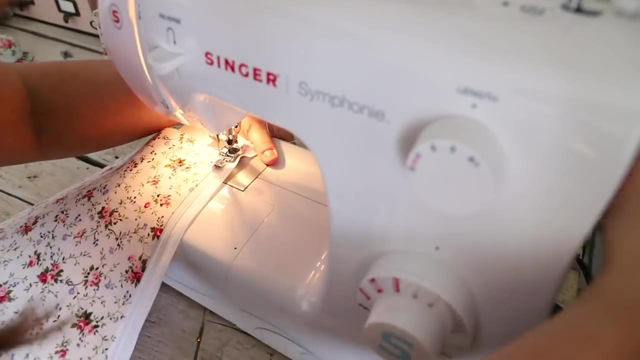 Once I have it ironed and pressed flat, I'm going to do a simple top stitch. This just stops the zipper kind of from bunching and the lining fabric from catching. so I always do a top stitch when I'm doing my zipper and it makes it look really professional as well. 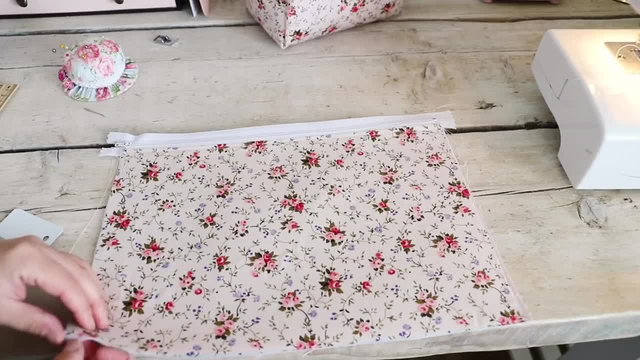 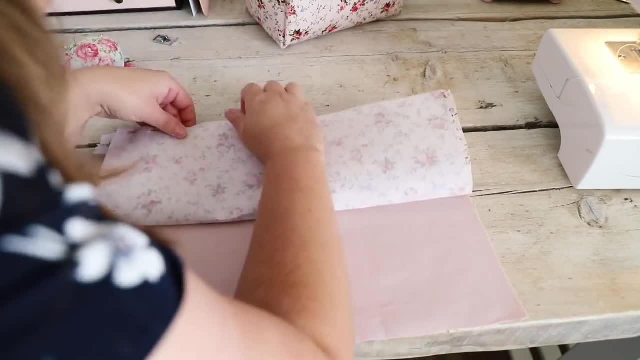 Once you have finished your top stitch, you are then going to work on the other side of the pouch, So your zipper is going to be facing the other way now and you're going to put the right side facing the zipper, and then you'll see me flip the lining and I'm going to have like: 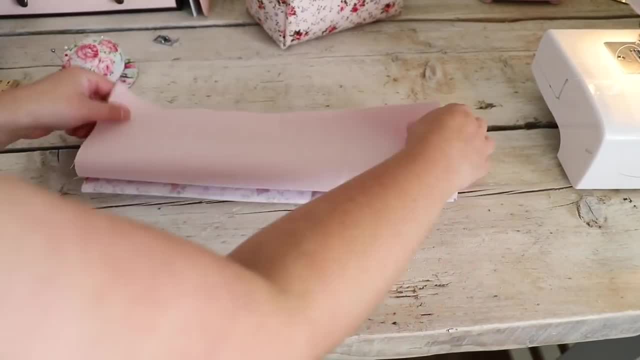 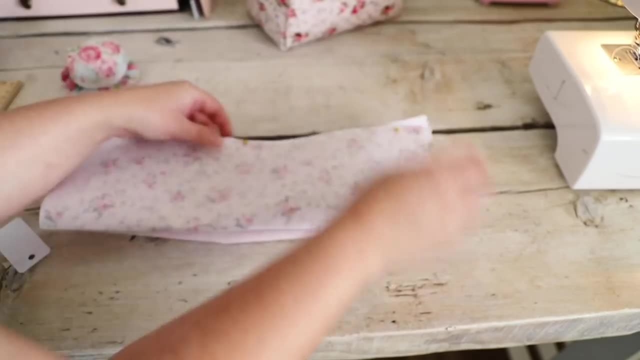 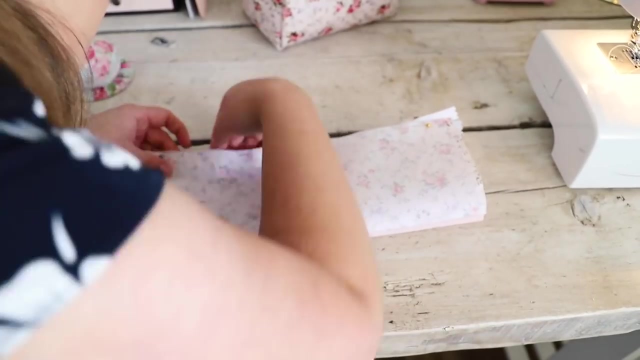 a sandwich. now I hope you can follow this when you're actually doing it in person. it makes sense. You are then going to take it to the machine and carefully sew straight down. Make sure to just use loads of pins if you're finding it a bit fiddly. definitely doing the. 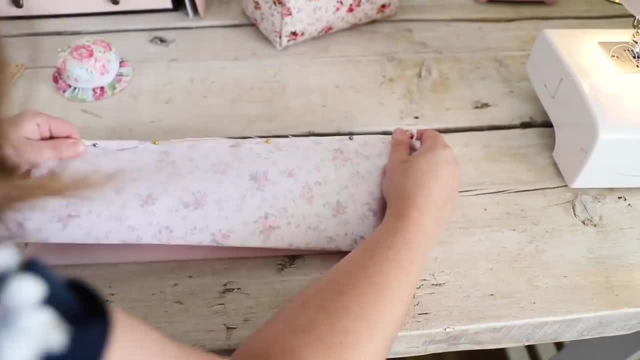 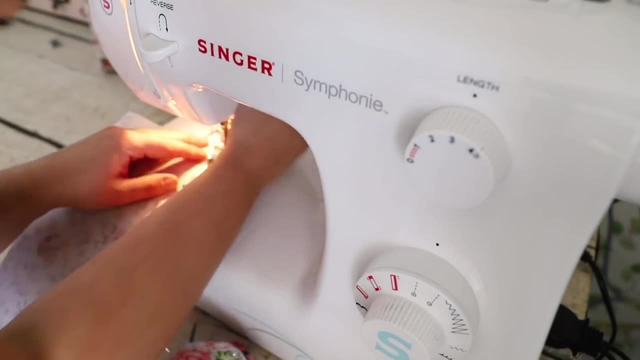 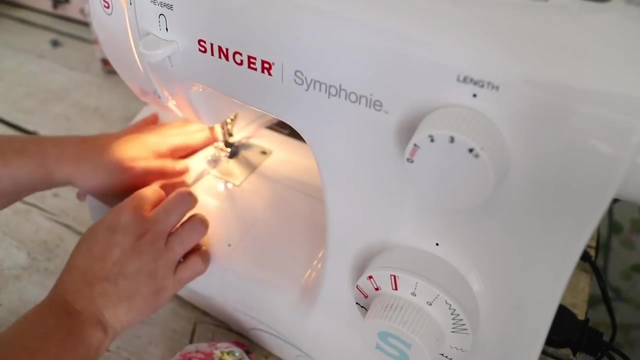 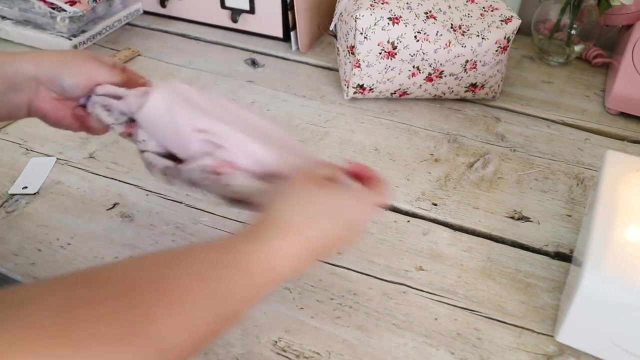 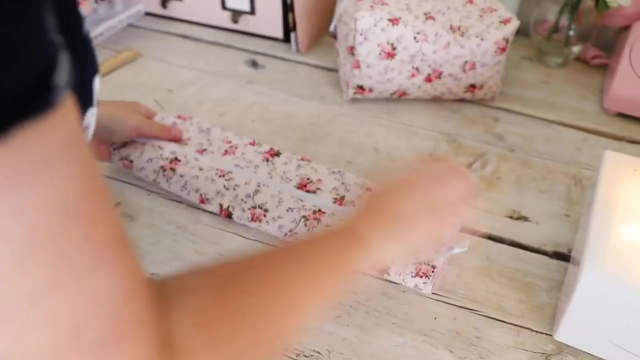 second side of the zipper is a little bit fiddly, but just persevere and it will be perfect. You can now pull your fabric through and you're going to have like a little roly poly tube of fabric. What you can also do is iron out the seam again and you can do a top stitch on the other. 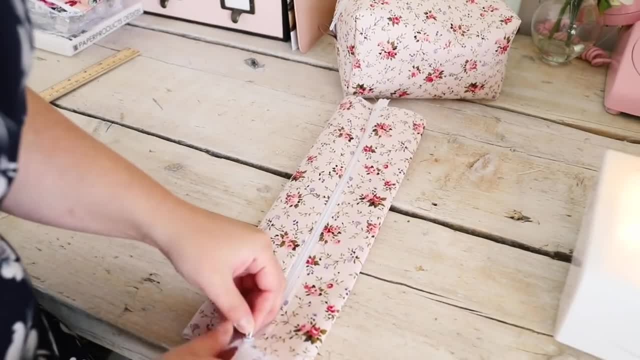 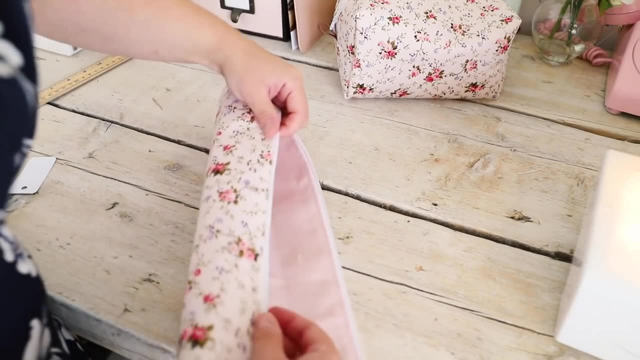 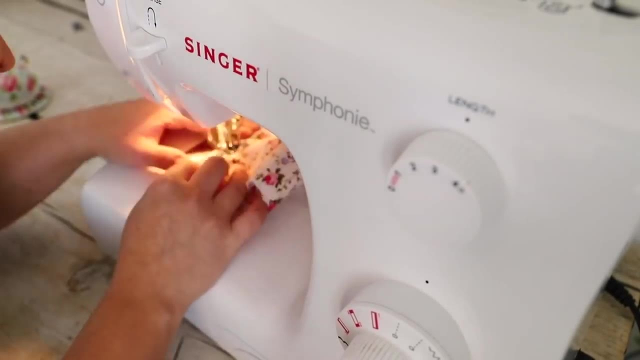 side. It is a little bit fiddly to do- You are just going to have to maneuver it into your machine- but it's definitely worth it and it will give you that nice polished finish. So you will be happy to know the hardest part is done. 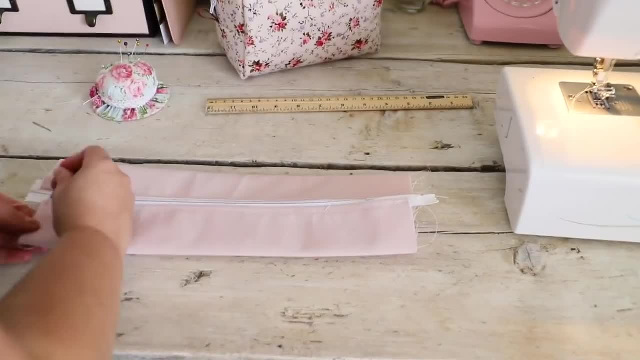 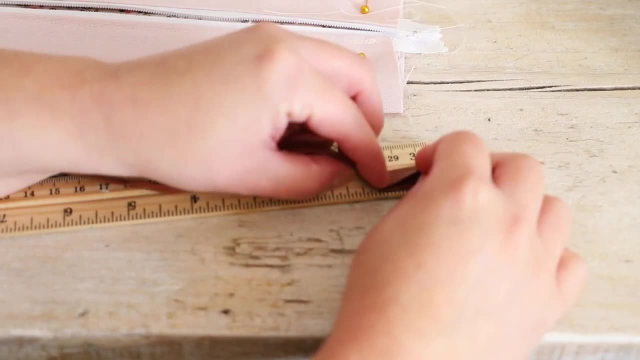 We are now going to box off the corners, and boxing off the corners will give you that nice boxy shape. We are also going to pop in some pull tabs so that it's easy for you to open your pouch and you have something that you can hold on to and pull. 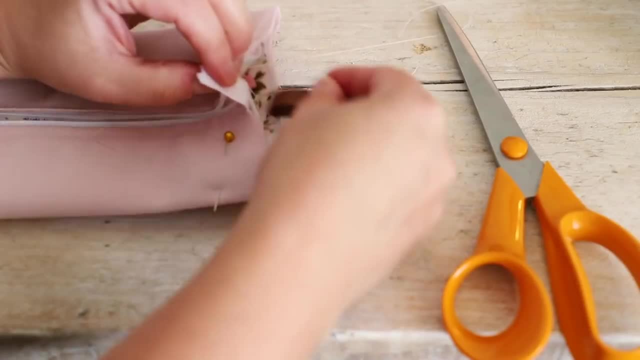 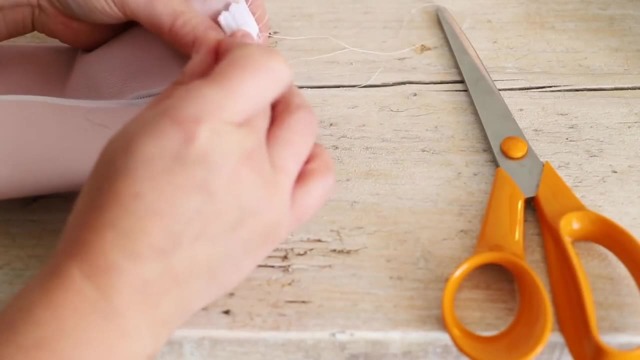 You can make fabric pull tags, but I'm just using some faux leather material and I'm simply popping it in right where the zipper is. I found the center of my bag and I'm just popping them in. If you have any excess fabric on the edge, you can simply trim it off. you'll see me. 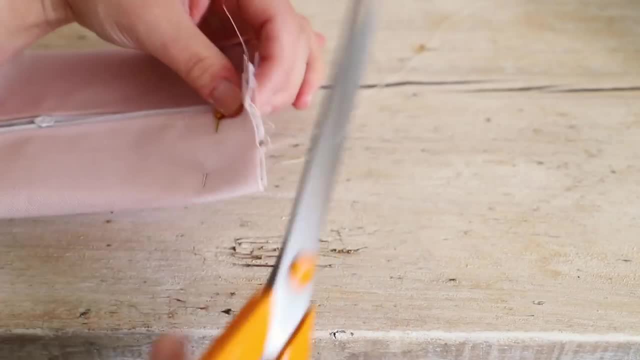 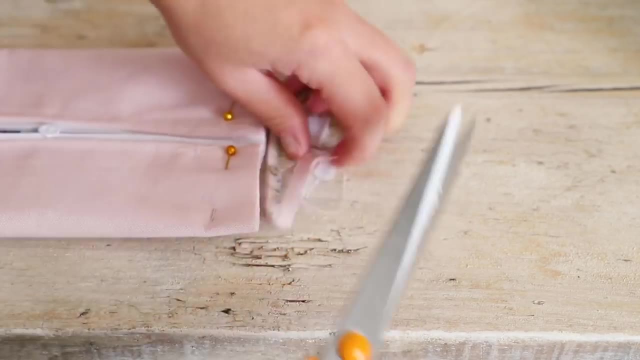 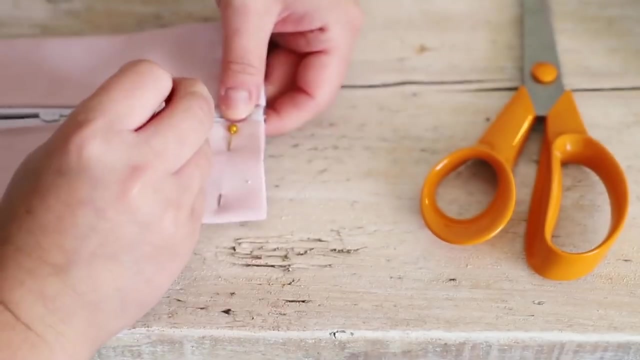 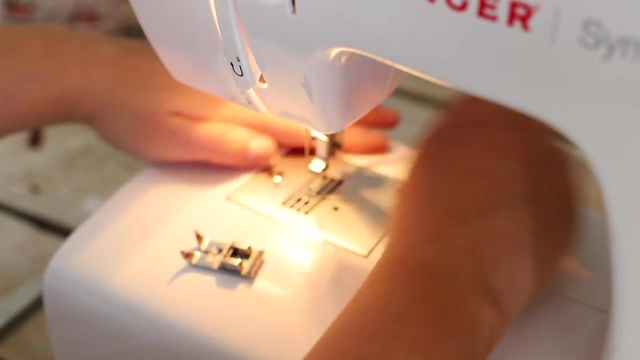 trim this off now in a second and that just gives me a nice even finish and there's no loose ends. Before boxing off my edges, I've just done two side stitches to close either side. I also just changed my zipper foot and put back on my normal foot, but you can actually 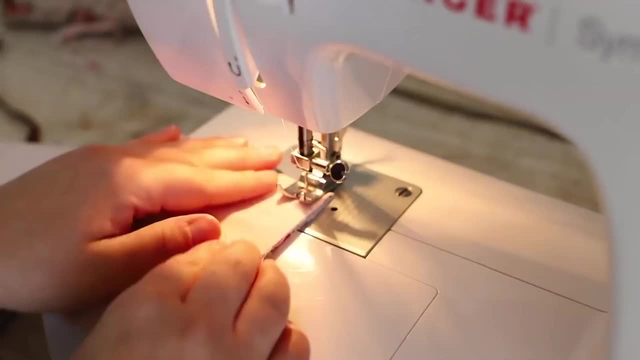 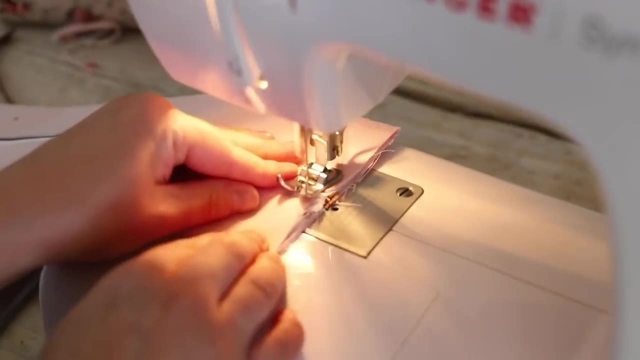 still use your zipper foot. It is a bit more fiddly, but you can just pop your old one back in. So two side stitches, Two straight stitches, and that is the sides closed. Don't forget to do a reverse stitch when you start and finish sewing. 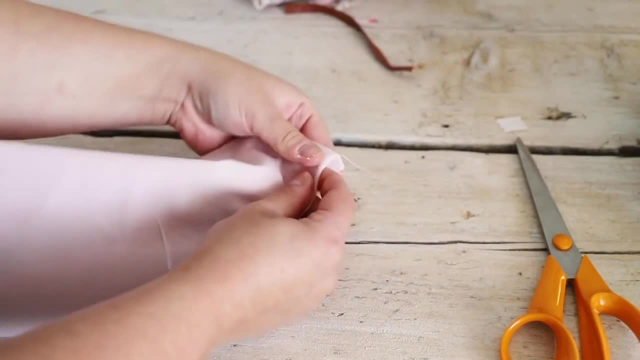 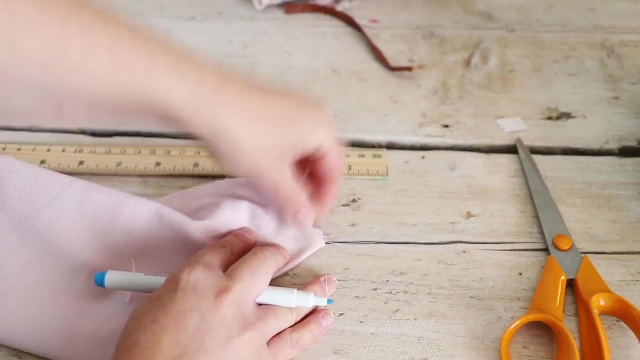 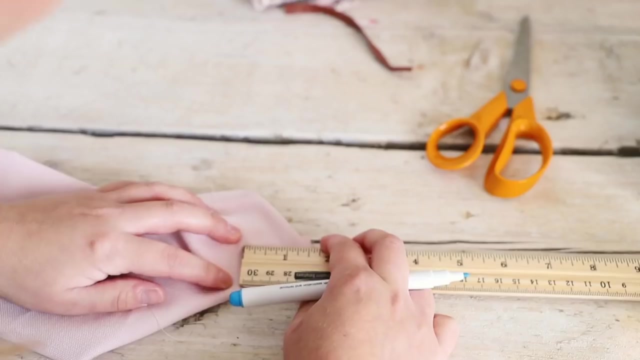 And now we are going to box off the corners. So you are going to do this four times because you have four corners. So you are going to find the point in the corner fabric. You're going to measure an inch. So for this one I used an inch, but I am going to leave measurements in the description box. 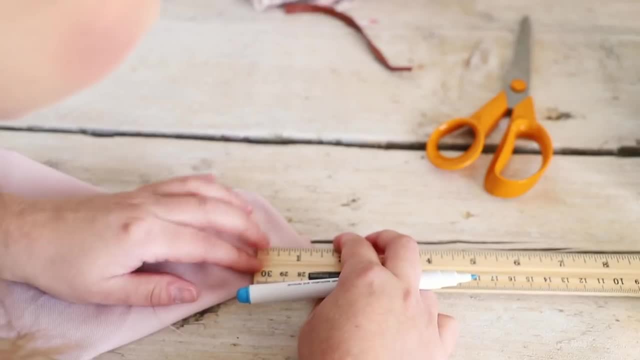 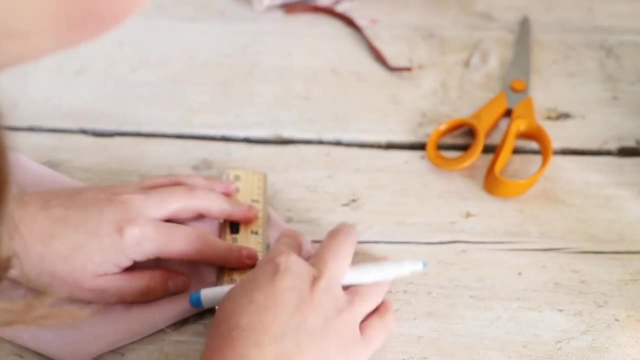 for another size and you're going to use two inches, But I'm simply measuring an inch, One inch from the point and marking it with a marker. This is a special marker for sewing. it's water soluble, so once you put damp water it. 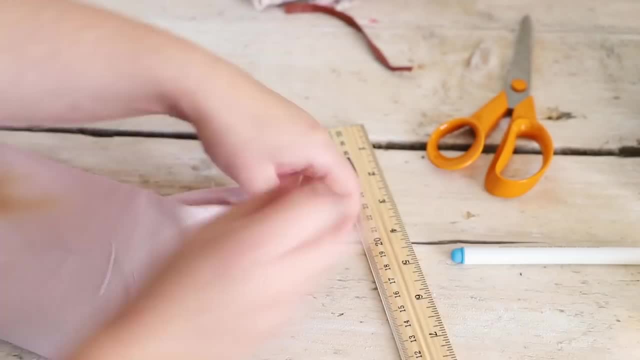 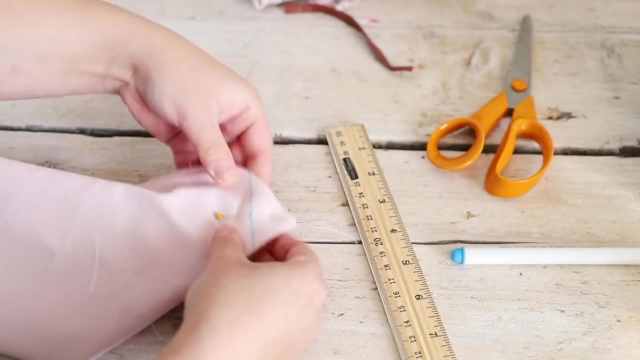 will disappear. So I'm just drawing a line, popping a pin in, because we are then going to sew that straight line and cut off the excess fabric, And I'm going to do this for all four corners measuring in one inch. drawing a line and 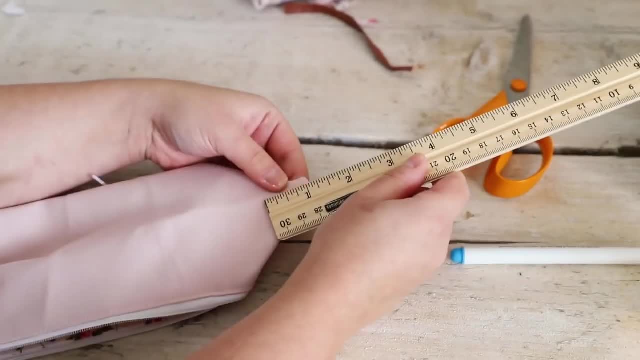 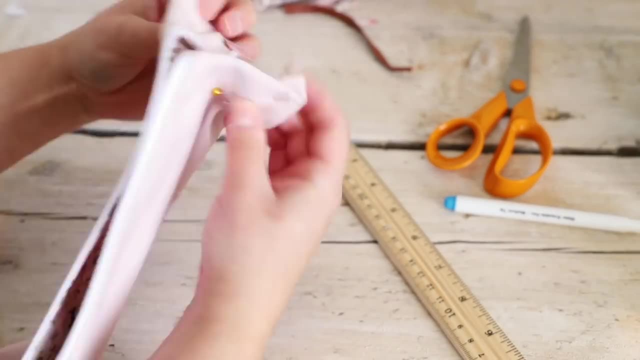 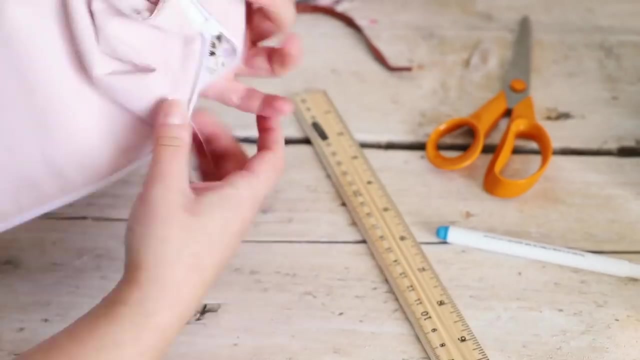 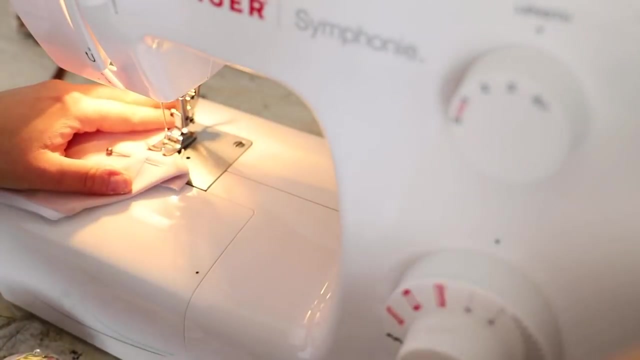 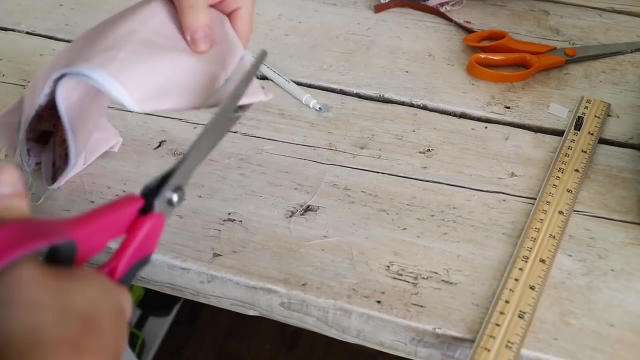 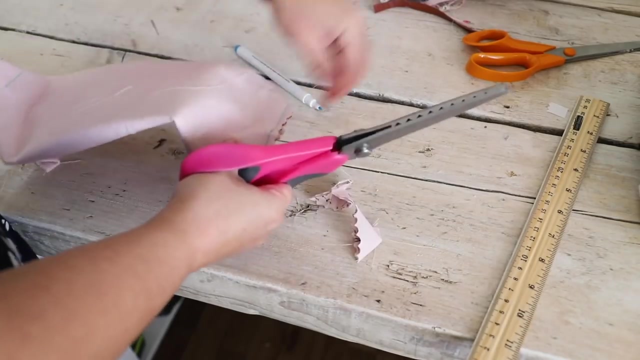 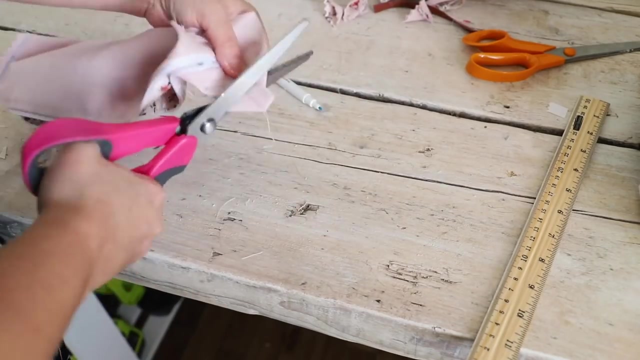 then sewing. Once you are finished sewing, you can cut off the excess fabric. I'm using a- I think it's called a pinking shears. I call it a pinking shears. I think it's called pinking- Basically the wiggly scissors, because this is going to be a raw hem and you are going. 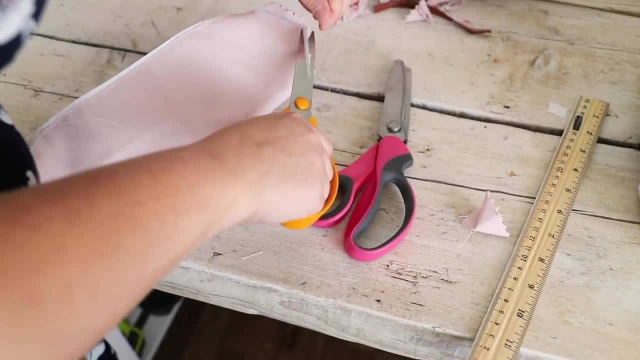 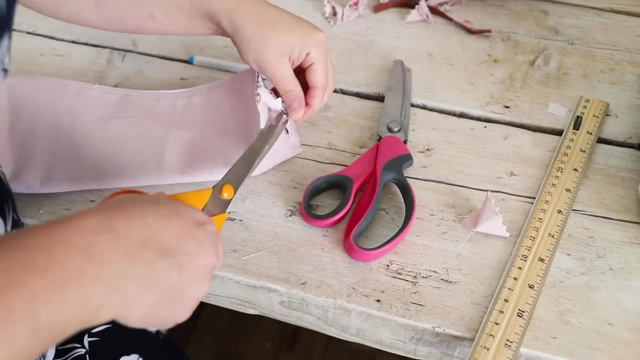 to see it inside of the bag. You're not going to notice it too much, So you can just neaten up any kind of loose threads, and you can also just remove the marker as well and tidy up, because we are finished our bag once we pull it through. 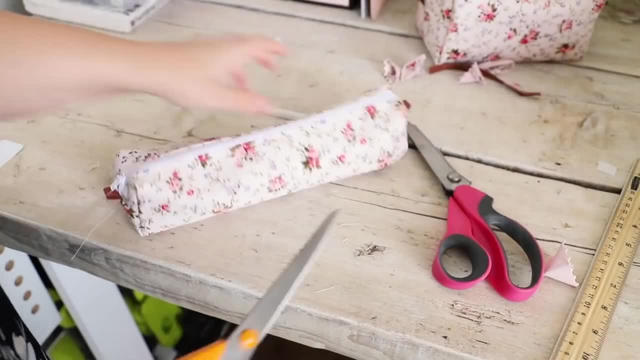 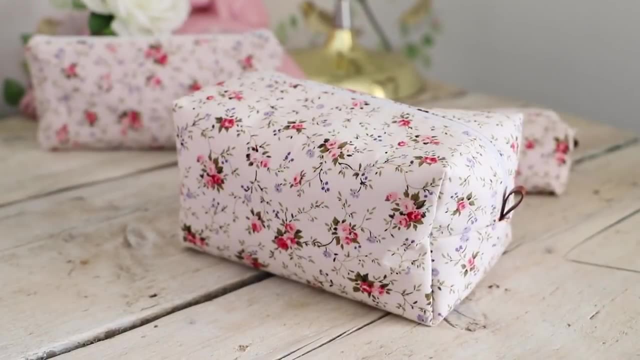 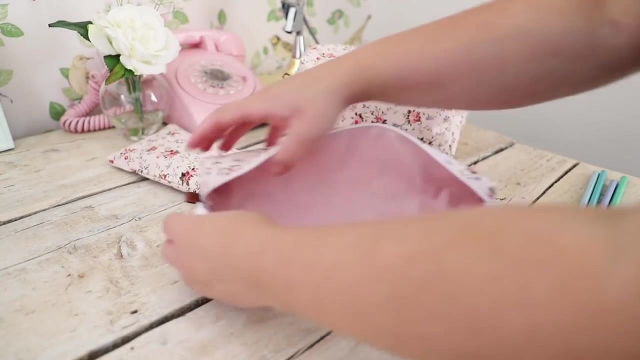 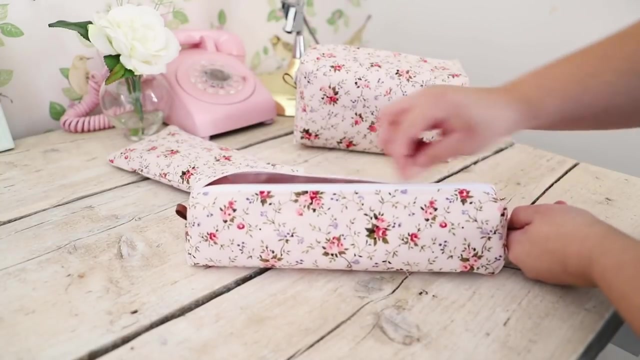 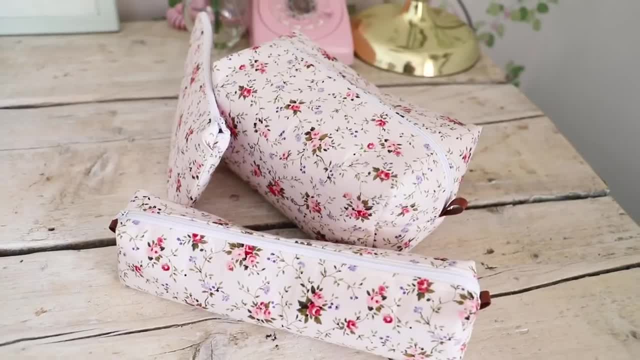 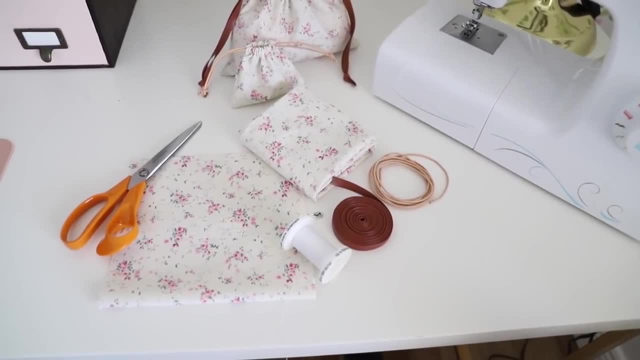 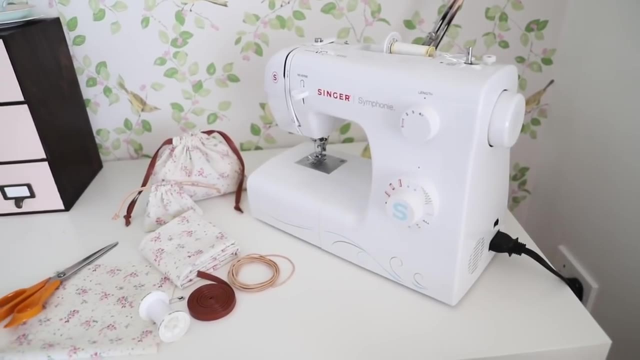 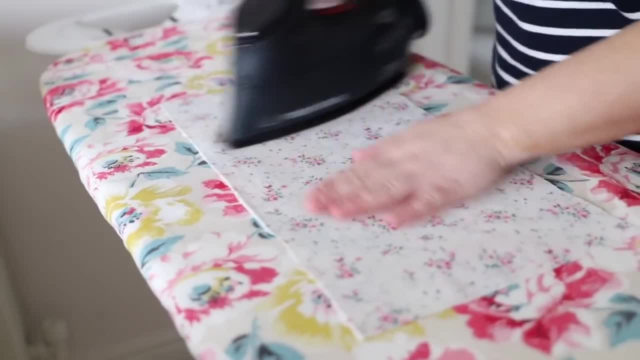 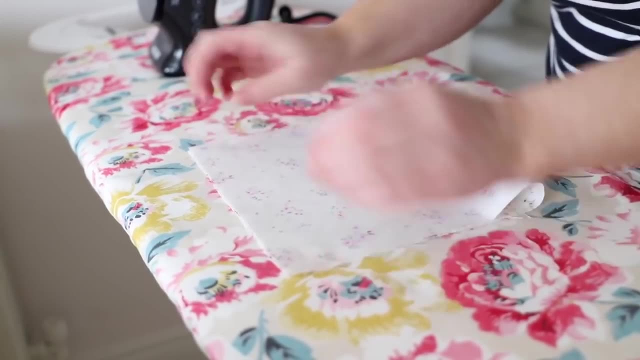 need your scissors, some thread. you're gonna need some twine or string for the tie parts and then your trusty sewing machine. So I started with a strip of fabric and I just ironed it to take out any creases. I then folded the right sides together and I folded down a piece to make a tunnel and 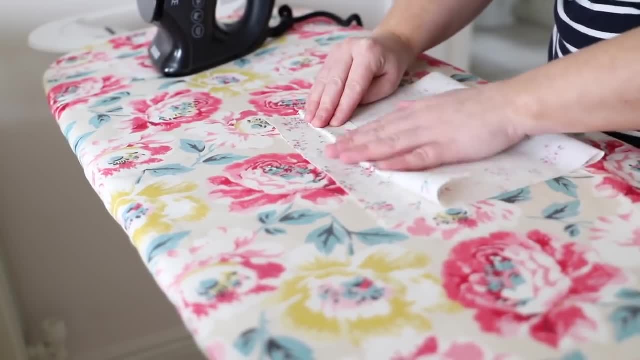 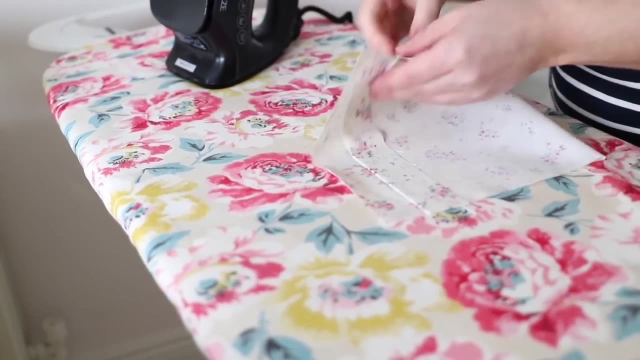 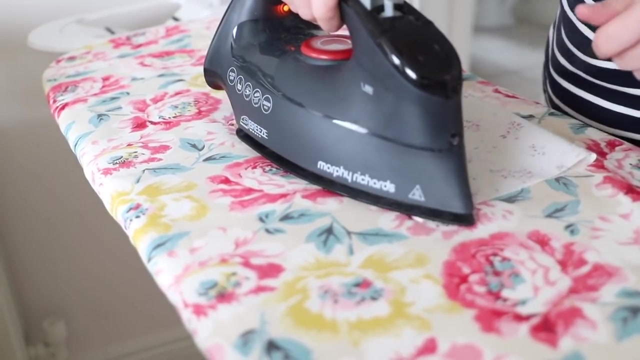 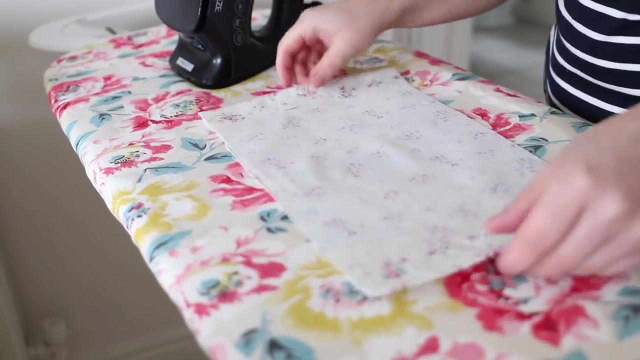 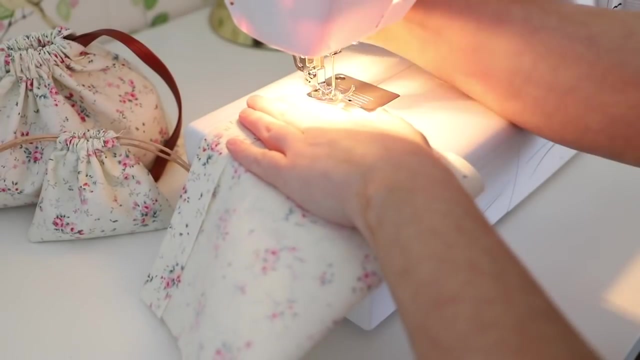 I ironed that flat. Then you're going to take it to the sewing machine and you're going to put a stitch on either side. You can see how I've done this in the next clip. When sewing, don't forget to do a reverse stitch at the start and finish of your stitching. 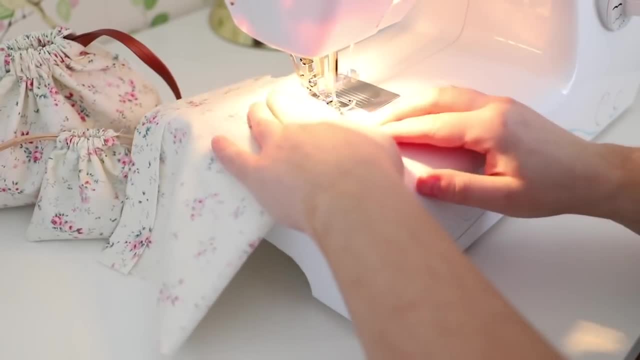 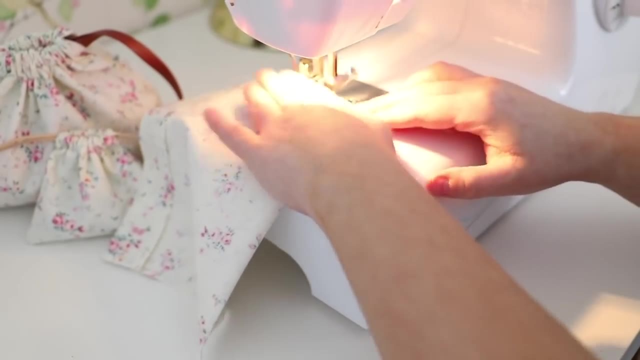 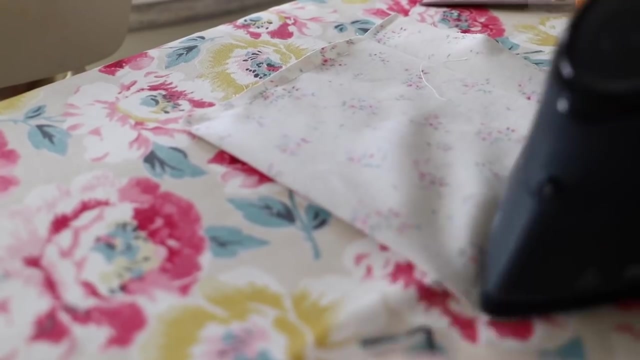 Especially if you're newbie. it can be easy to forget to do a reverse stitch, but this is really important as it stops your sewing from unravelling. Once I was finished sewing, I ironed my seams out flat. Sometimes, when you're new, you can forget to iron out your seams, but this gives your 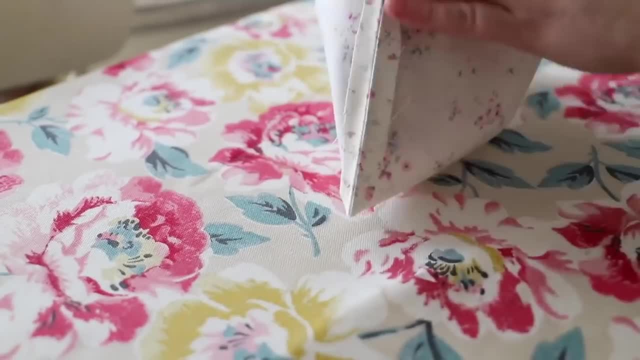 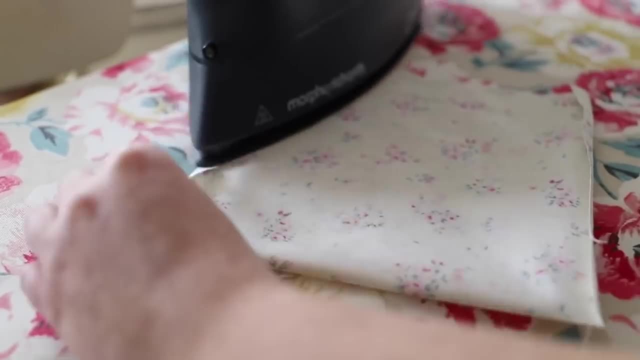 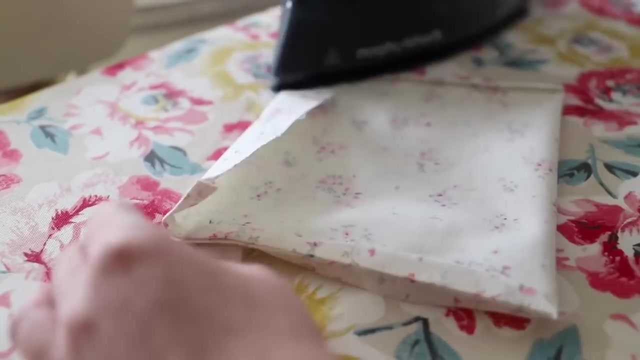 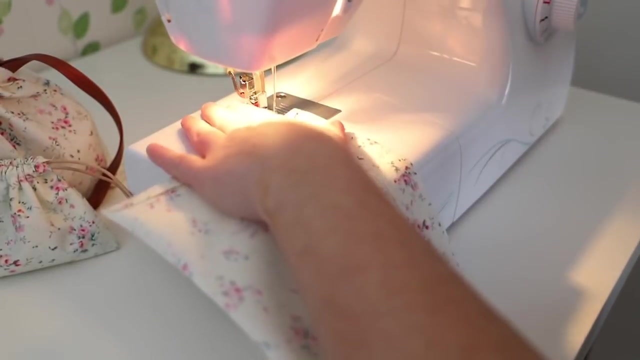 piece a really polished finish. It makes it hold. It's shaped better as well. so iron out your seams. I'm now just sewing my tunnels closed, so I'm going to do a straight stitch down, leaving obviously a gap on the inside, because this is where you're going to put your piece of. 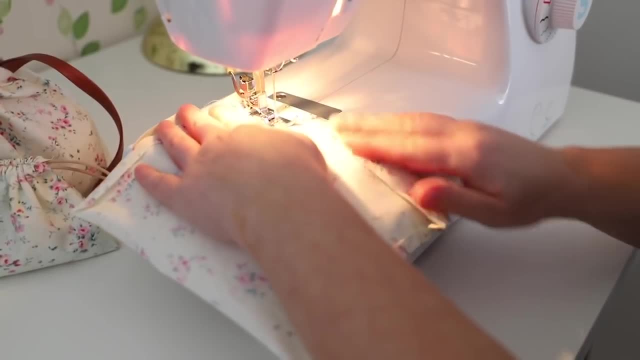 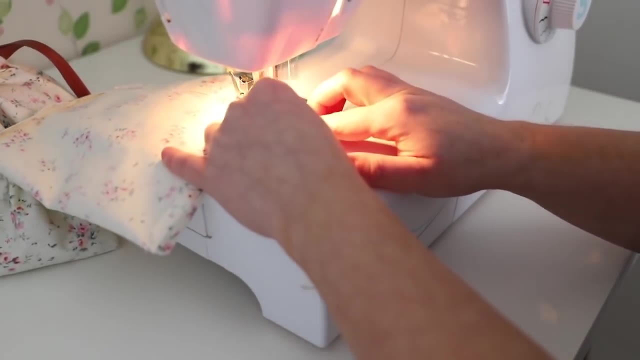 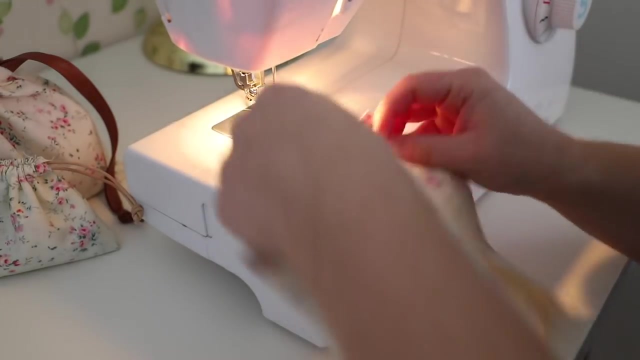 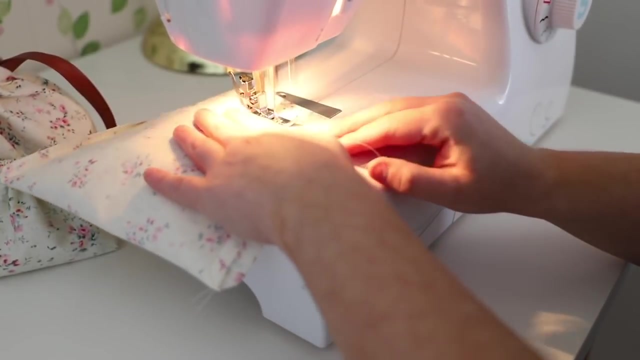 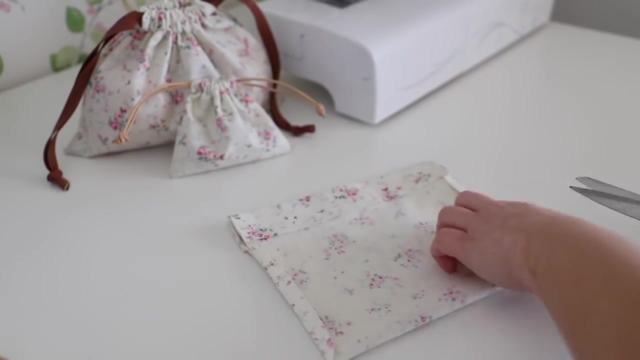 string in to make your tie Okay. Also, don't forget to do a reverse stitch at the beginning and end of your stitching to keep it nice and secure and in place. I'm now just going to turn it right side out and I'm going to trim off any excess pieces. 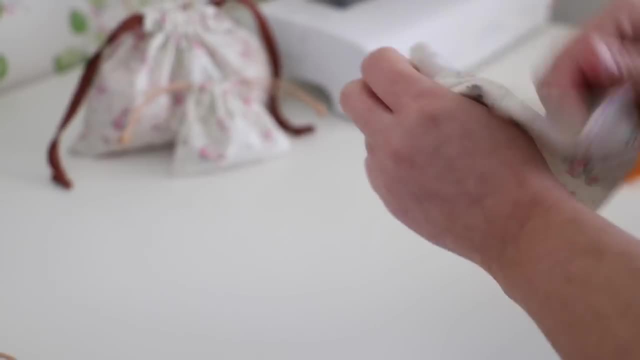 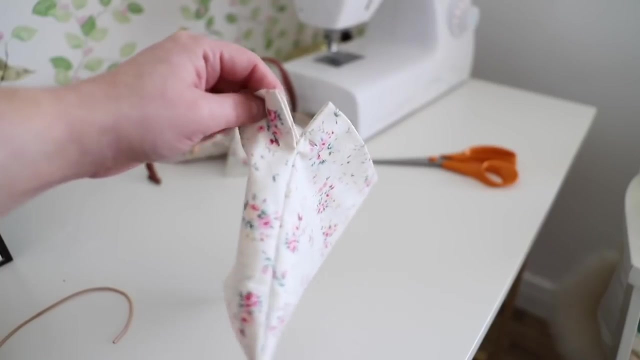 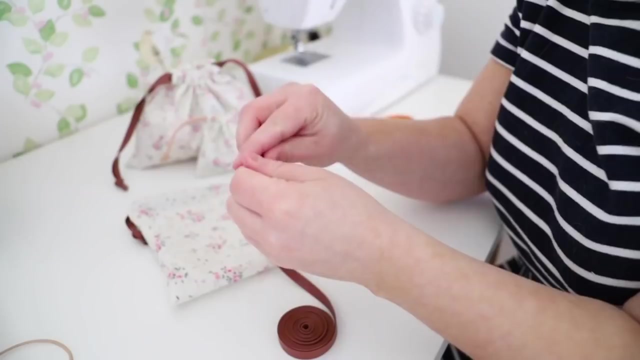 of threads, or whiskers as I like to call them, You can really poke out the corners to get a nice sharp point on them. and now we're going to get ready and we're going to pop our thread through our little bag. 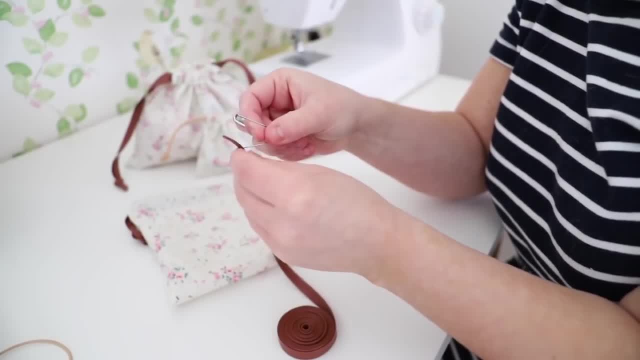 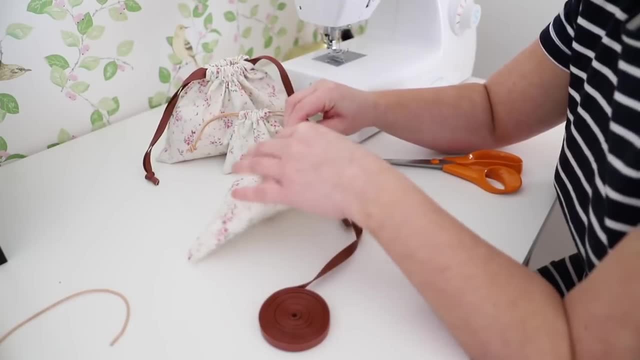 I'm using a safety pin to attach my cord to the safety pin and then I'm going to push the safety pin through the tunnel And this is going to bring my string through the tunnel. Okay, I hope this makes sense and you'll see by how I'm pulling it through in the video. 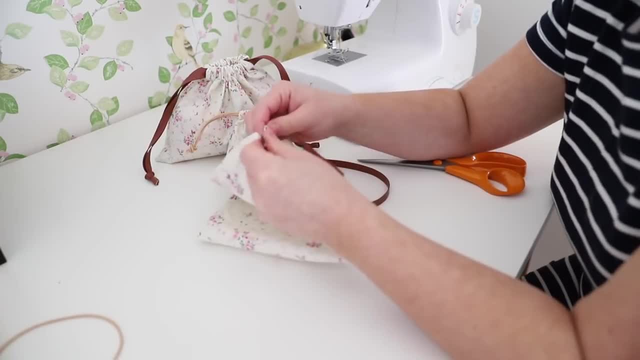 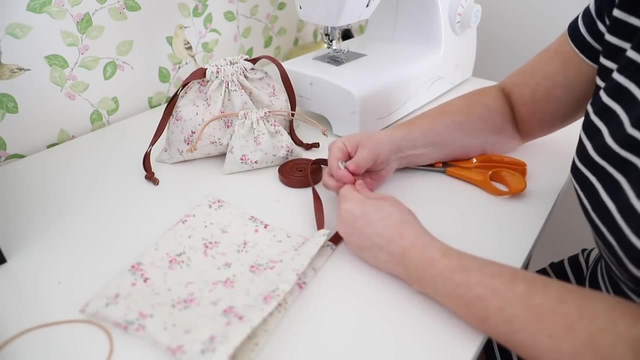 Once you have pulled it all the way through, you're going to bring it around the other side and you're then going to secure it with a knot, and you're then going to do the whole thing again, but just on the opposite side, and you're going to secure that with a knot. 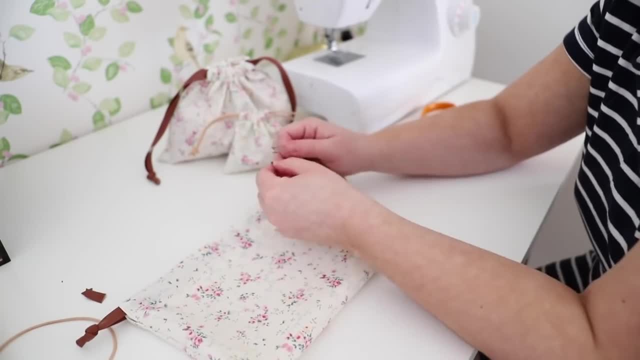 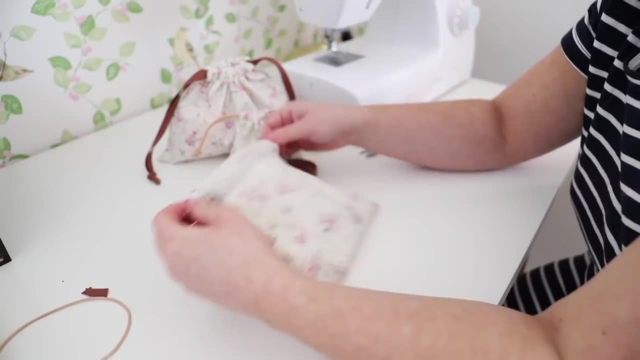 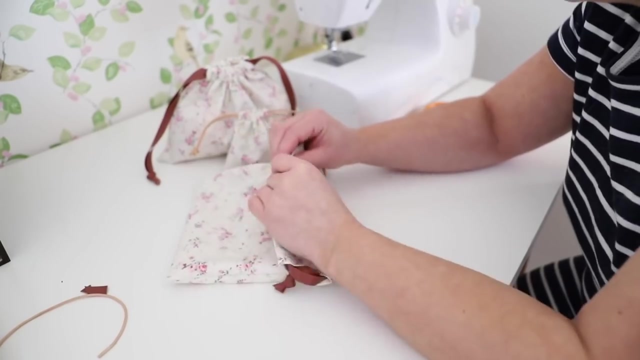 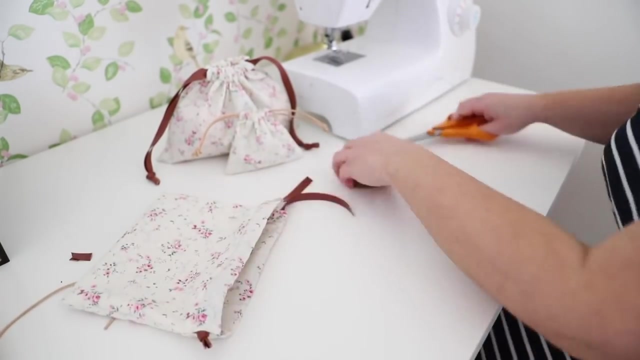 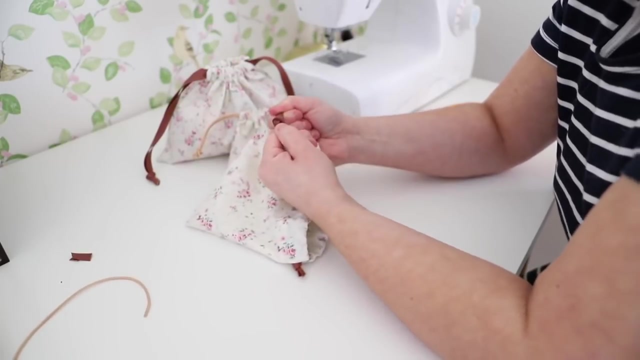 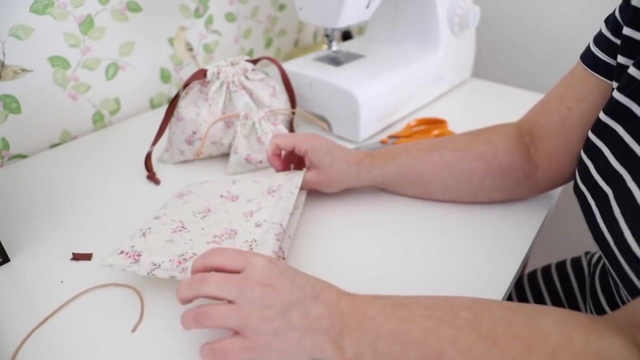 as well. Once both sides are threaded through, you can trim off any excess, and then you can give it a test and pull it and see how the bag assembles, and then to loosen it, you just gently pull it and loosen it. 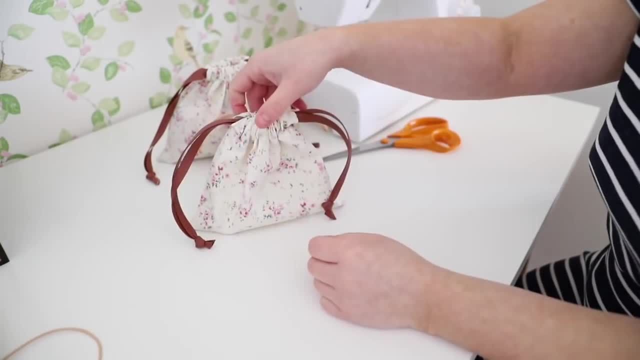 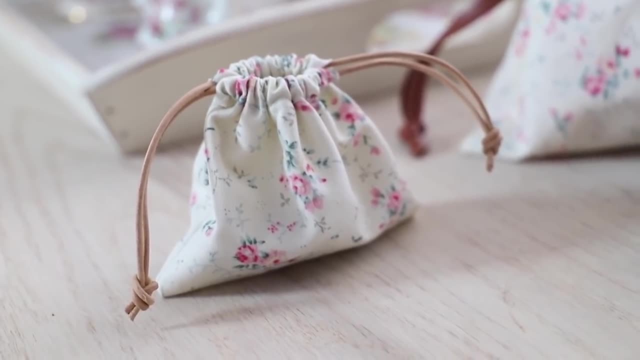 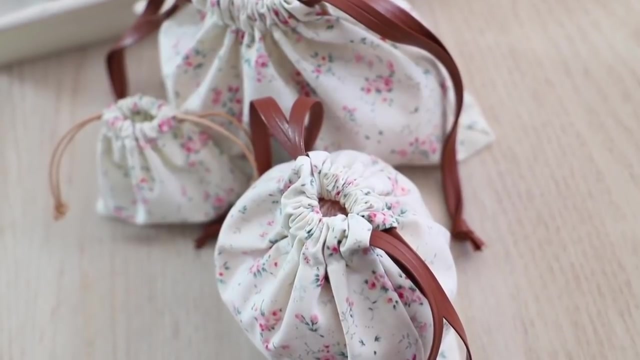 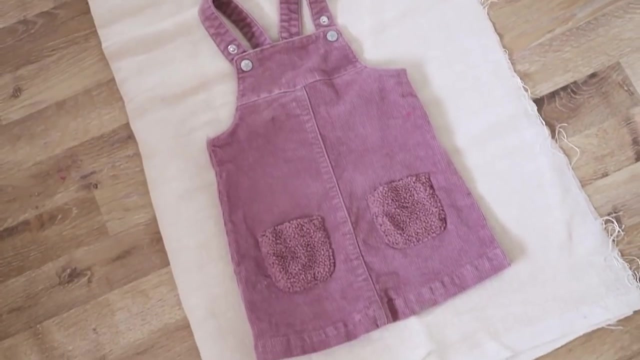 Okay, I'm going to be making an apron from drop cloth fabric, so you know that painter's fabric that you can get in most DIY shops. I'm going to be making an apron from drop cloth fabric, so you know that painter's fabric. 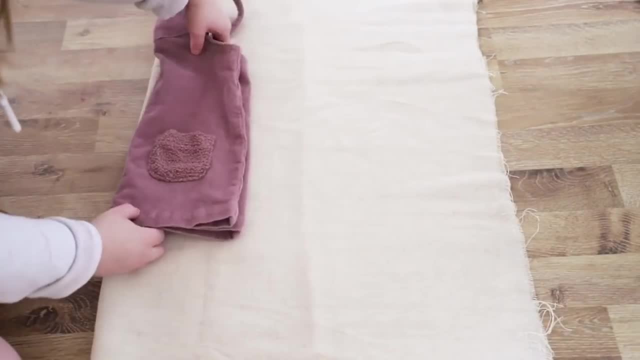 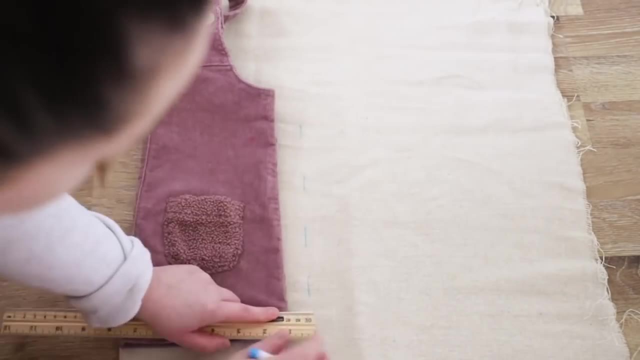 that you can get in most DIY shops. And because my niece is so small, I'm going to start where her's and I'm going to use her little pinafore as a template. So I'm measuring out an extra 1 inch all the way around, and then the same with the bottom. 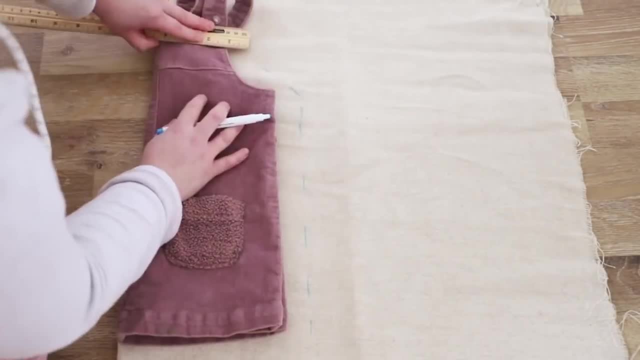 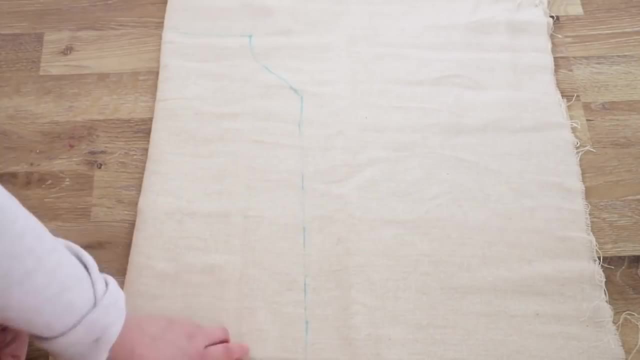 and then the sides, and that's going to give me a base template for her apron. I have placed this on the fold, so, as you'll see, when I cut this out, it's on the fold and it will open up into one large piece. 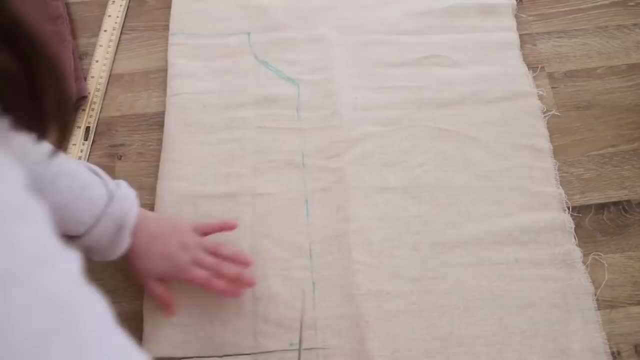 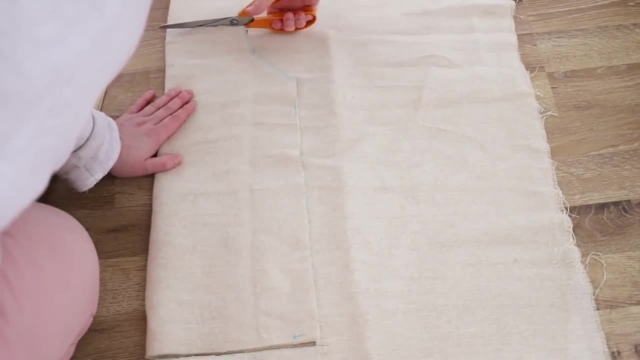 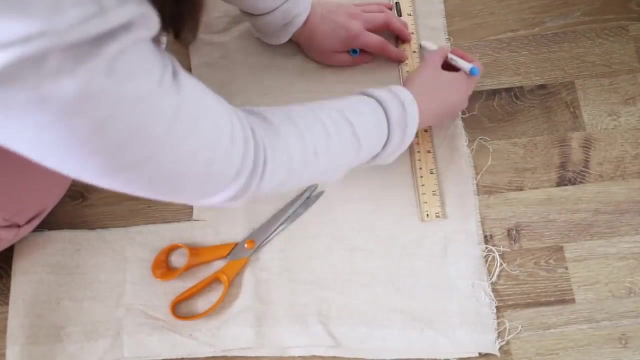 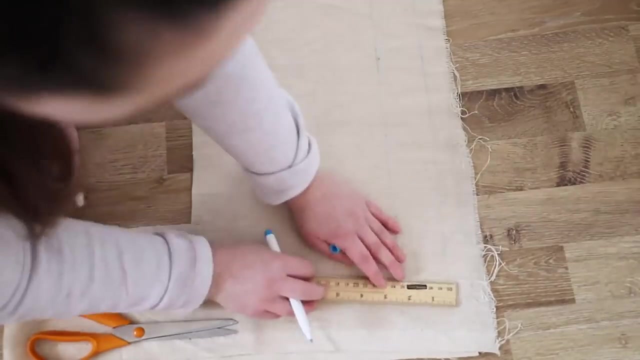 and then I add a pocket as well. I used her straps as a guide. so the straps that were on her little pinafore, I used them as a guide and I just doubled the measurements and I cut out four pieces because I'm going to have four strings. 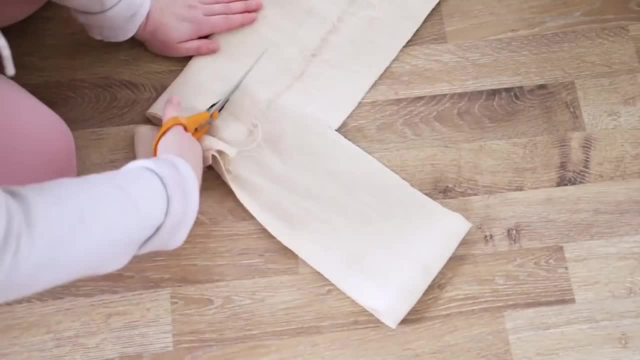 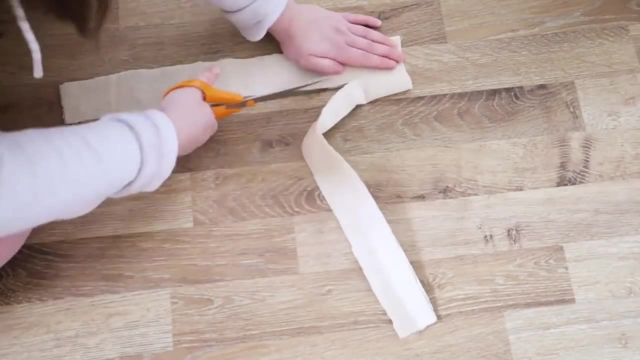 Once I have the four strings cut out, I'm going to take them to the ironing board and I'm going to show you how to assemble them. Now, the drop cloth fabric is a bit on the frayy kind of side. it's a bit fiddly, so you. 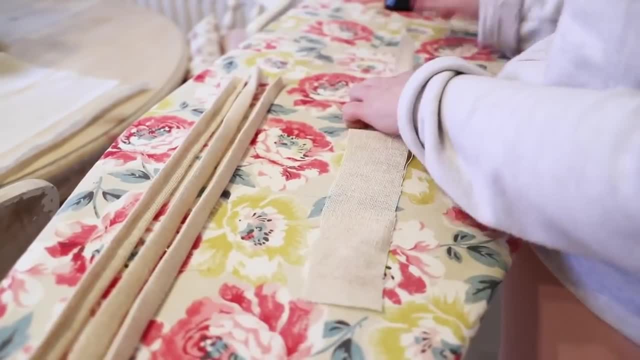 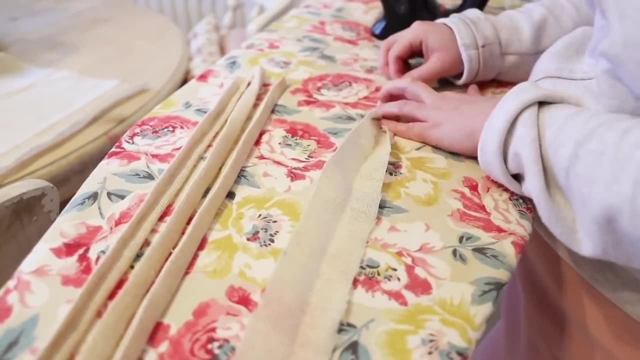 can cut them a bit thicker if you want to, because they are a little bit difficult to iron. I fold them in half and then I fold them in quarters. basically, I fold it in half and then I fold the halves in on themselves, fold it again. 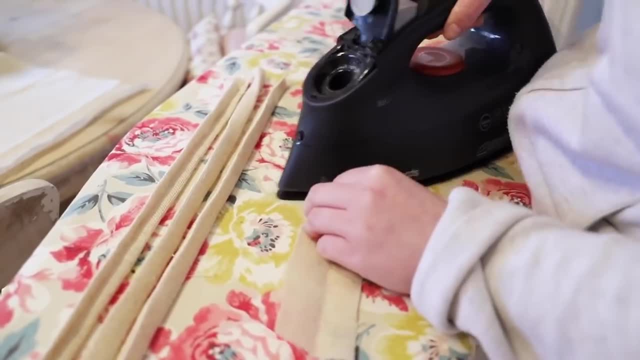 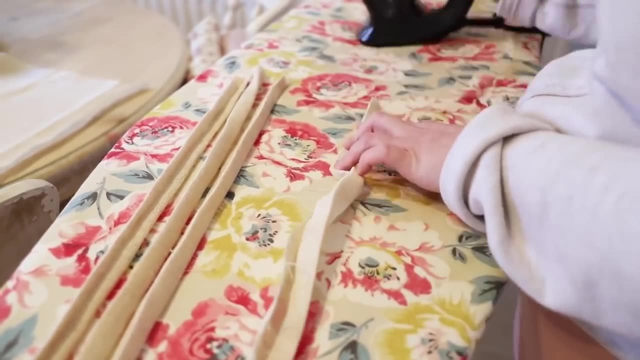 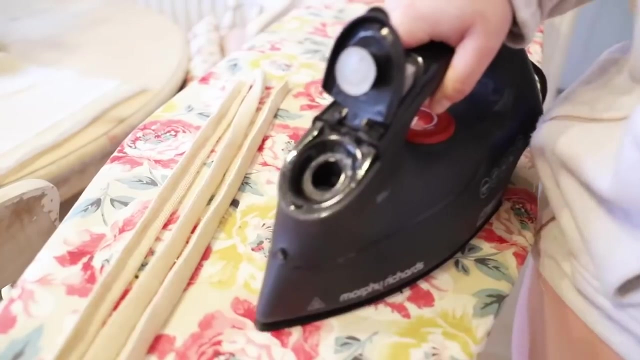 That gives me the perfect fold to create the strings and then I do a straight stitch down either side. I hope by looking at this video you kind of get an idea of what I did. I also folded in the raw edge on one end of the tie and the other end you can leave the. 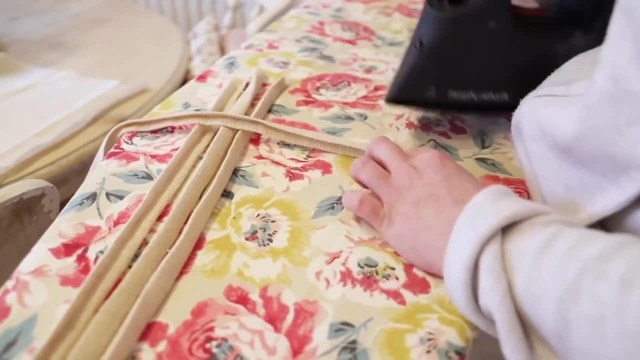 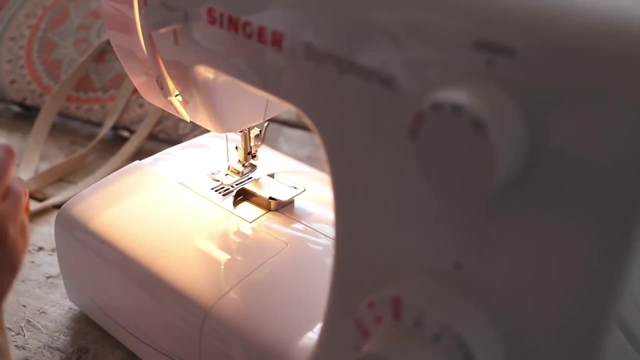 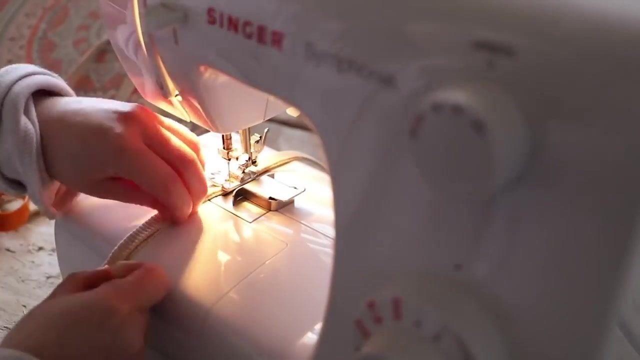 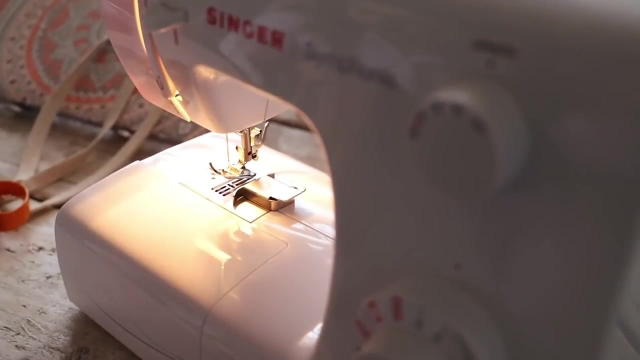 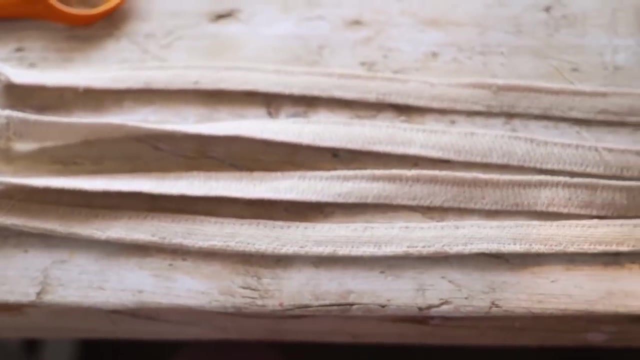 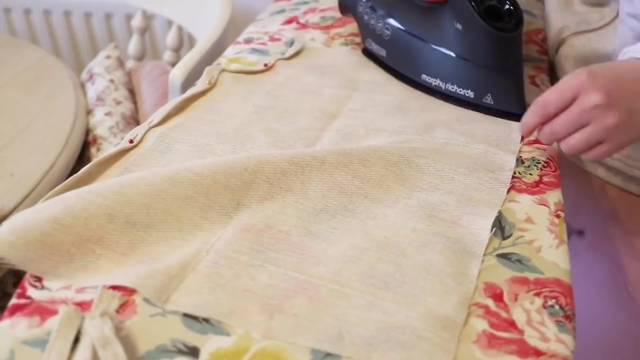 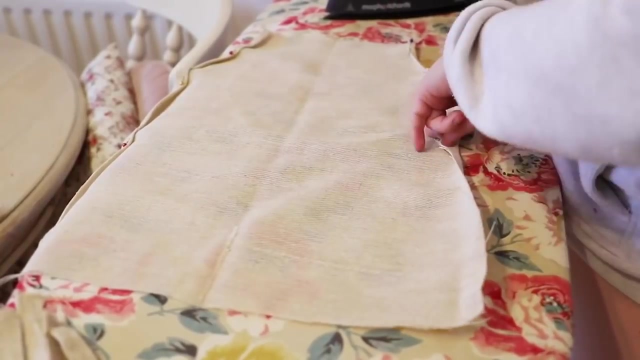 raw edge free, because that is going to go inside of the apron. Now we're going to work on the body of the apron and I'm simply hemming all the way around. so I'm folding over once, I'm ironing, and then I'm folding over a second time and I'm just 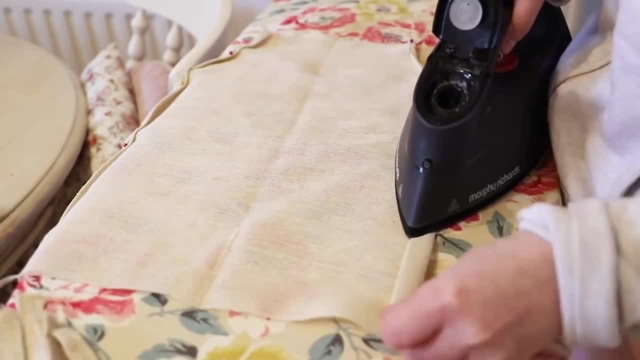 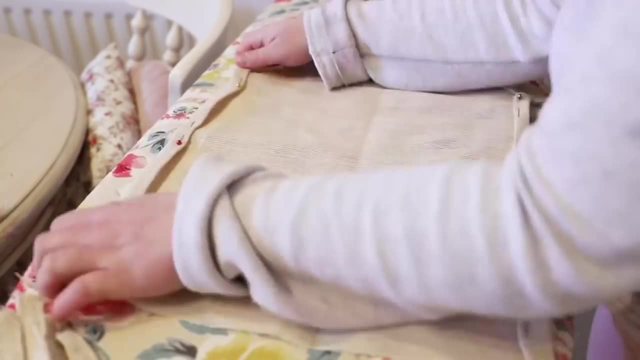 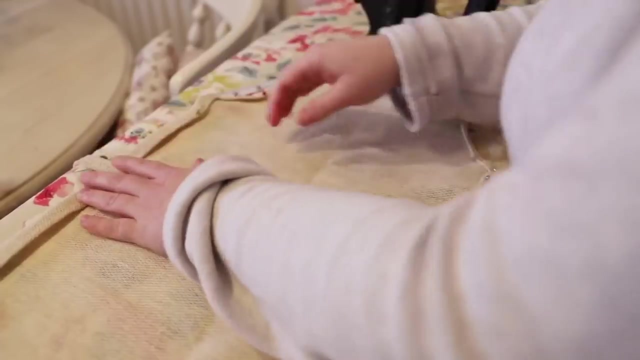 pinning it into place and now we're going to place the ties or the strings into the body of the apron. So I'm going to measure down so that it's even on both sides, and you'll see how I put the string in and then flip it over, add a pin, and I do this on both sides and I just 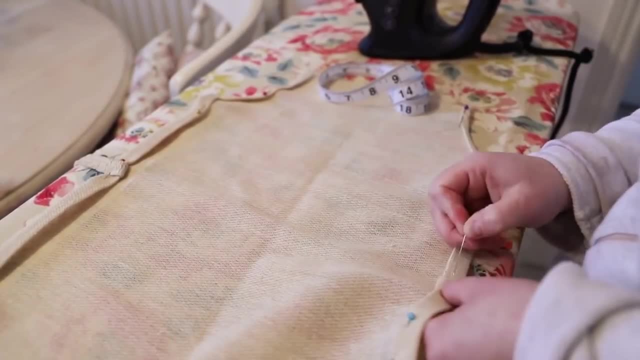 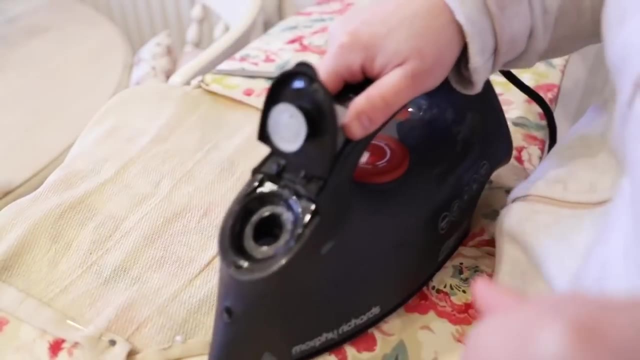 measure down to make sure that I have both of the ties symmetrically placed- And I'm also going to do that- on the neck of the apron. I'm going to add the ties in the same kind of place and when you do your stitch all the way around your apron, these 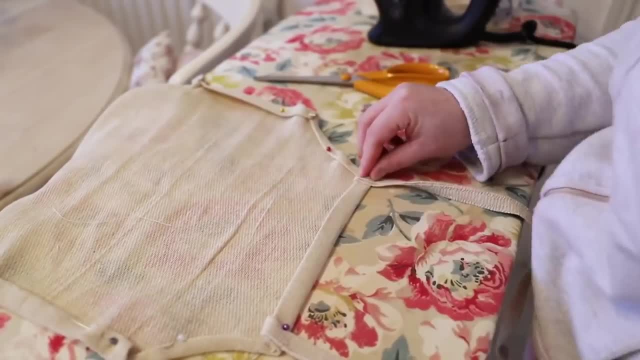 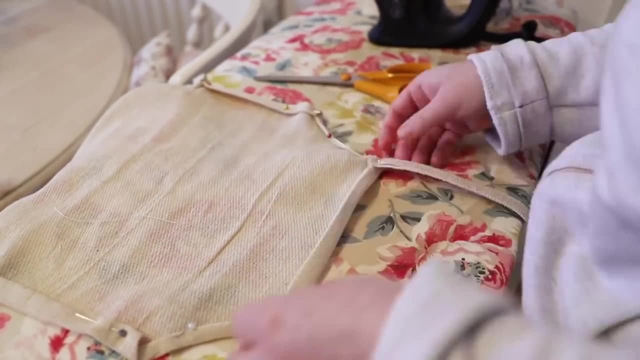 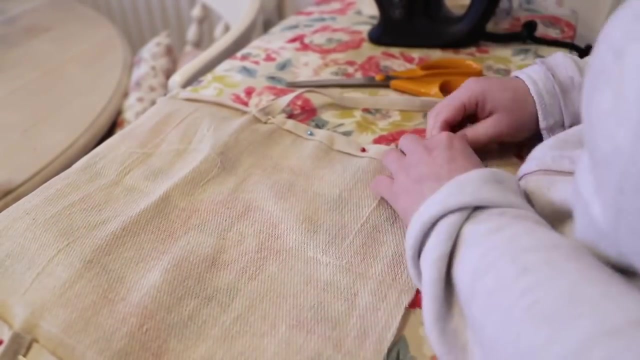 are going to be secured into the apron, and you can also do a reverse stitch on each tie just to make sure they're really secure. Now mistake number two of the day is coming up. you'll see, now I melted my measuring tape, and I'd love to say that that's the first time it happened, but it's not normally. 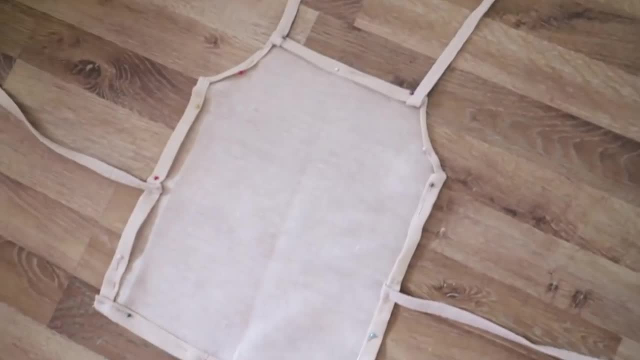 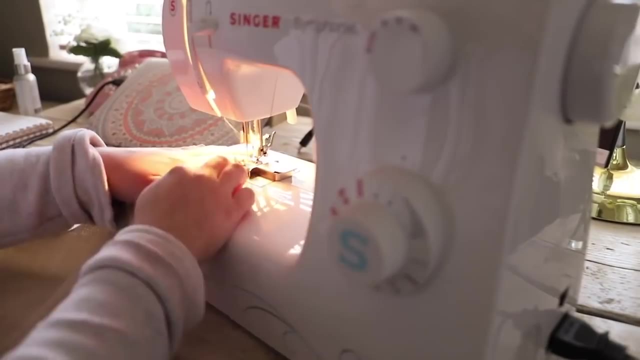 if I'm not melting the measuring tape, I'm cutting it. Another thing to note as well: ties may not be practical for young kids, which I kind of realised as I made it, but I know Lily is kind of fine when it comes to the strings. 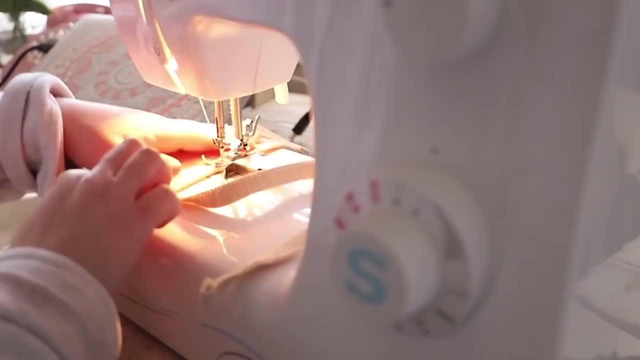 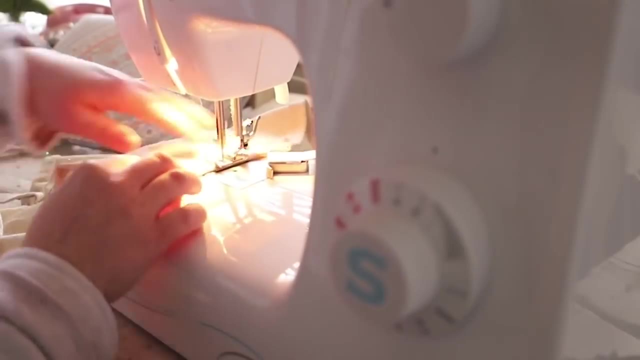 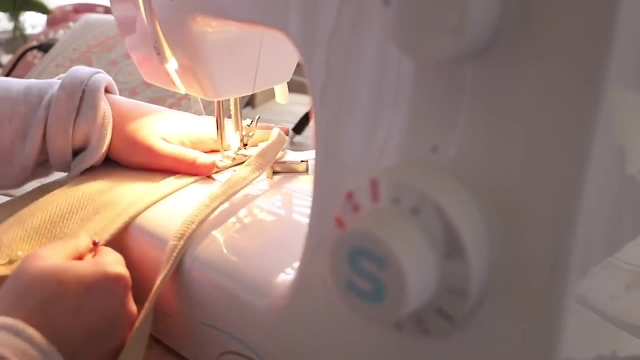 but velcro might be better for kids, especially around the neck. So if you are making this for, like, a younger child, maybe consider having velcro instead of knotting it. but I purposely made these strings extra long so that they could kind of be loosely. 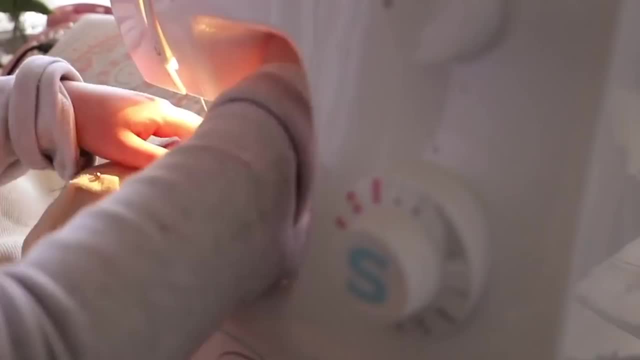 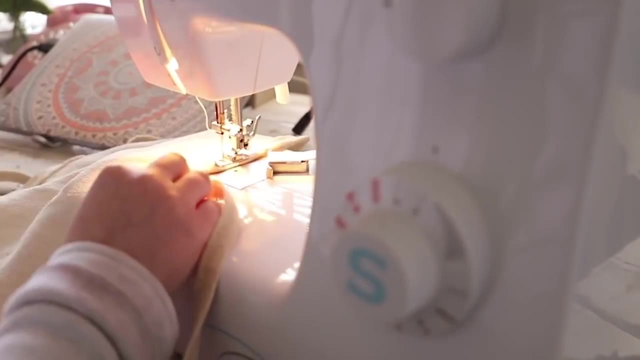 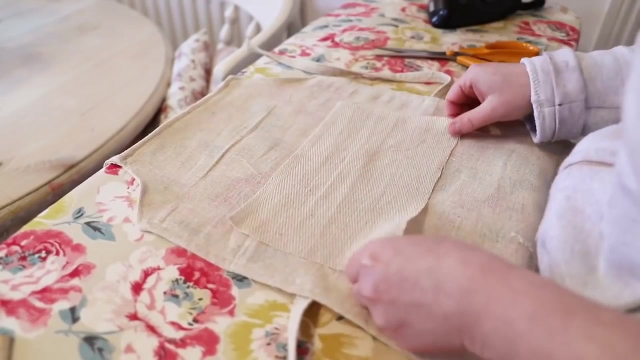 tied and that they wouldn't kind of be like a choking hazard. but just bear that in mind that for younger kids, maybe like a velcro strap for the strings, might be handy and safer. When I had made this I realised, girl, this needs a pocket, we need somewhere to put the. 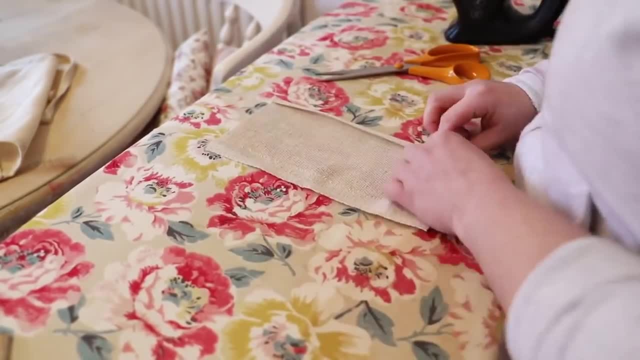 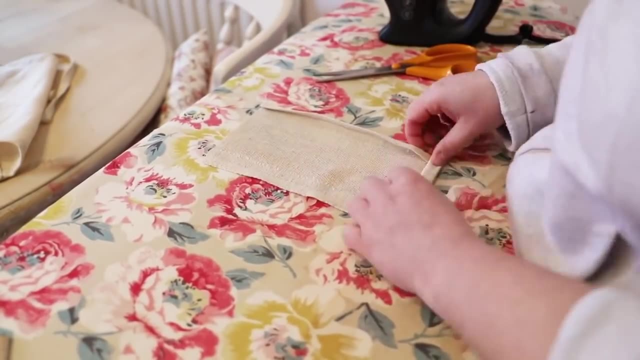 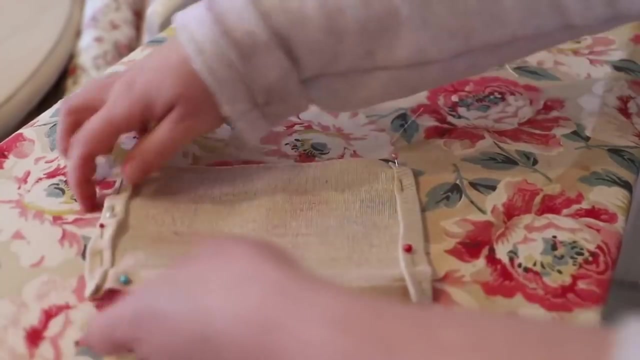 paintbrushes. so I popped the pocket onto the apron. so I just folded in the raw edge on three sides, found the centre of the apron, and then I popped the pocket on and pinned it in place, checked it, gave it a little eyeball make sure it was ok, and then I just 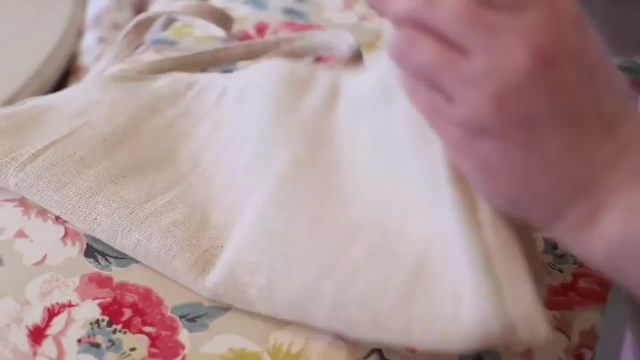 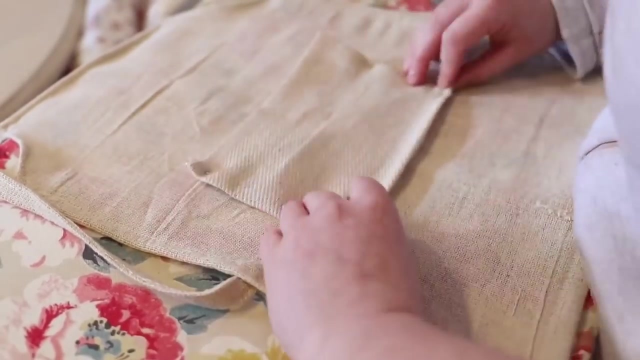 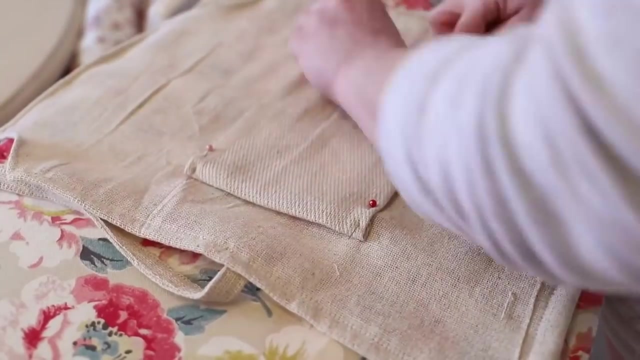 stitched all the way around and don't forget to do a reverse stitch at the first and last stitch To make another apron. so for my nephew Jack, he's much bigger so I just extended the pattern to his measurements. so I just added a couple of extra inches to the length and a couple 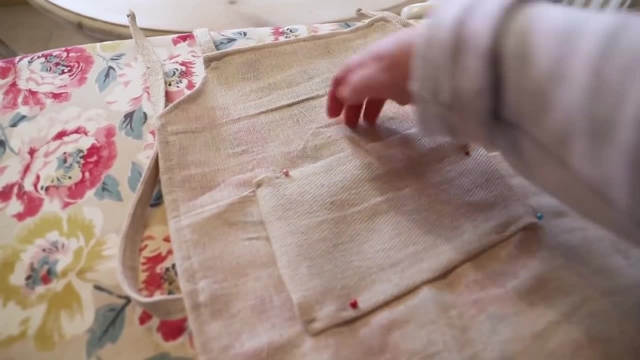 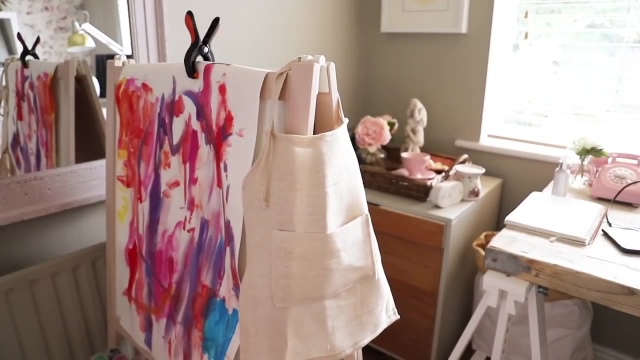 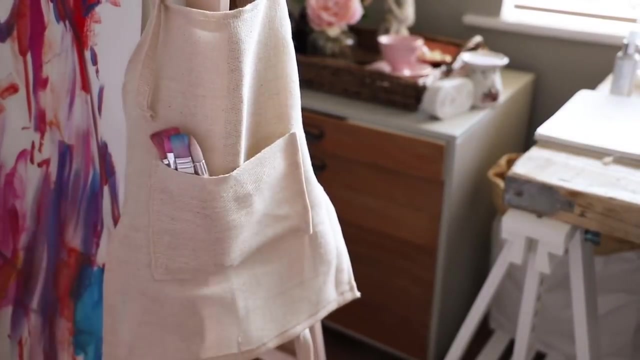 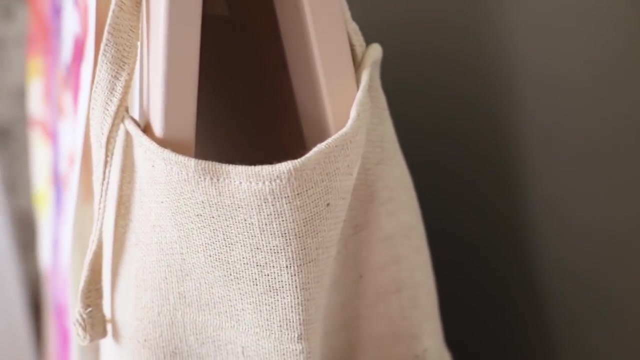 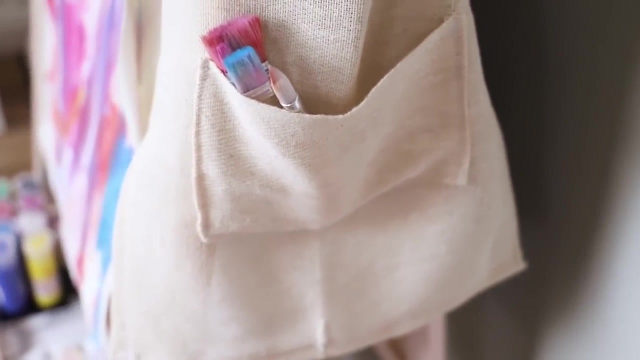 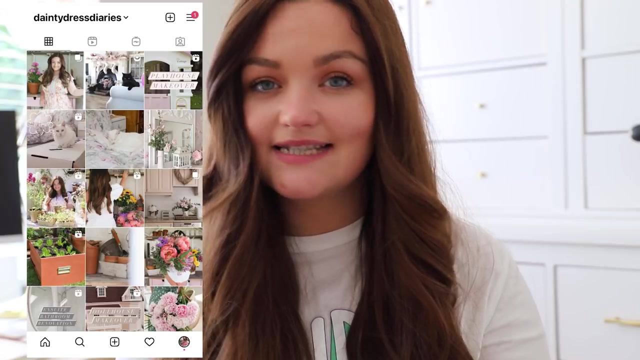 of extra inches to each side and then I used this as a template. So once you kind of make one template, you can use that as a base for making other ones in bigger sizes. I hope you got some inspiration from those sewing projects. do tag me on Instagram or. 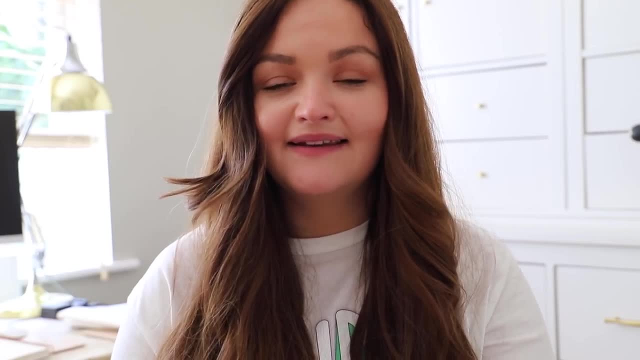 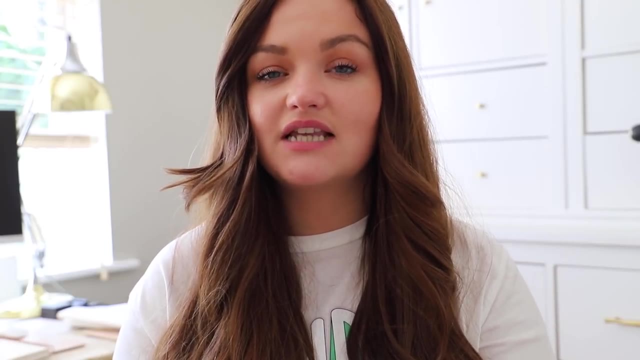 you can share your projects via email through my blog as well, and let me know if you got creative and does it work for you. Thanks for watching. Please do share this video if you know any kind of newbie sewers that you think would enjoy this. sharing is caring, and don't forget to subscribe cheeky thumbs up and I'll see.